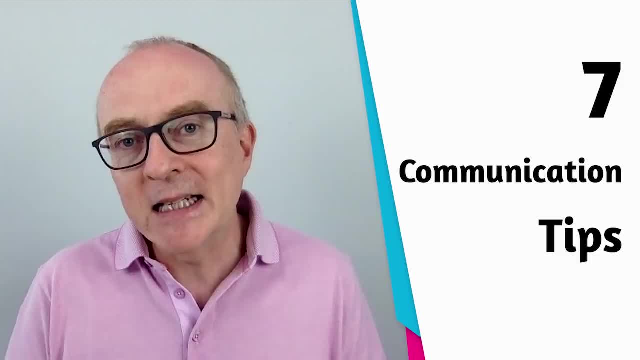 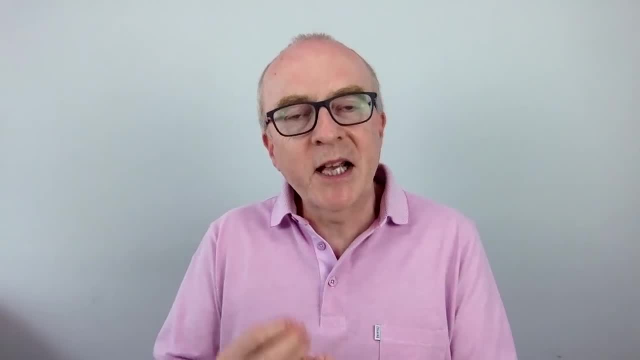 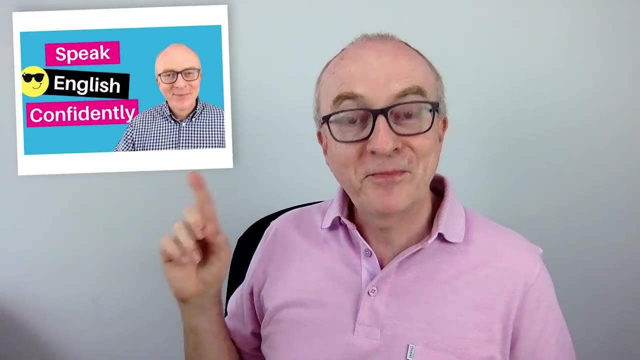 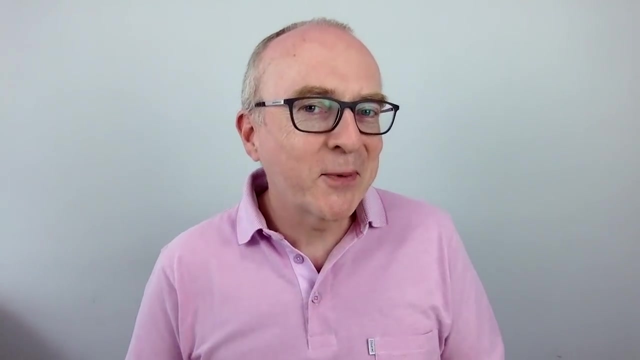 seven tips for you to improve your English speaking skills. in English, Remember right, I think communication it's a skill, it's like a muscle that you need to develop, A bit like confidence. Do you remember my last video about confidence? Well, it's something you need to develop over time through practice. A great place to practice. 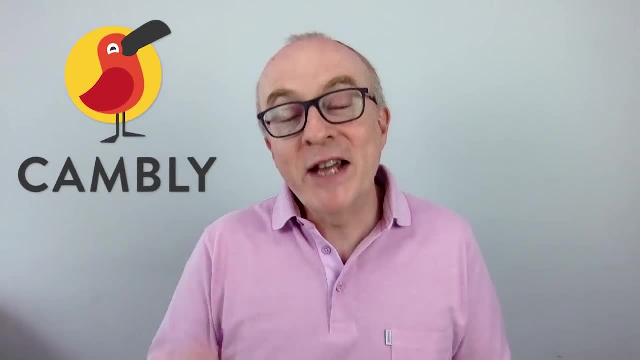 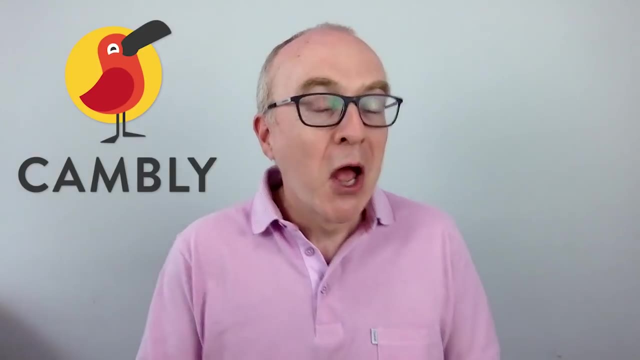 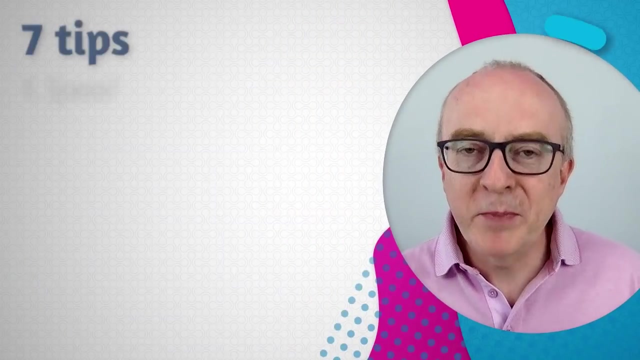 I think, is Cambly. Cambly have got native English speaking teachers who can help you practice English and develop awesome communication skills. More about that later, But today the seven tips I've got are the following: Speed- How fast you should speak. 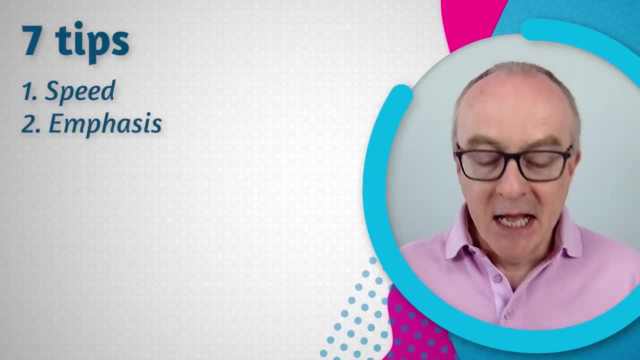 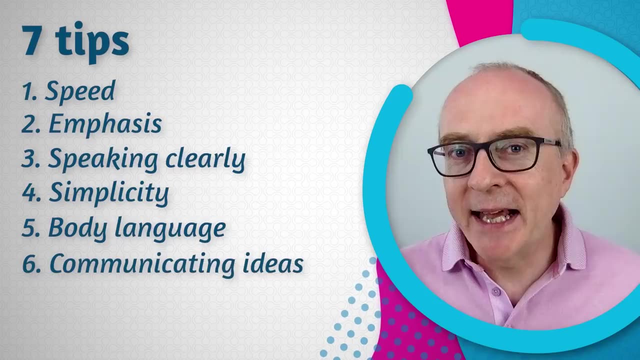 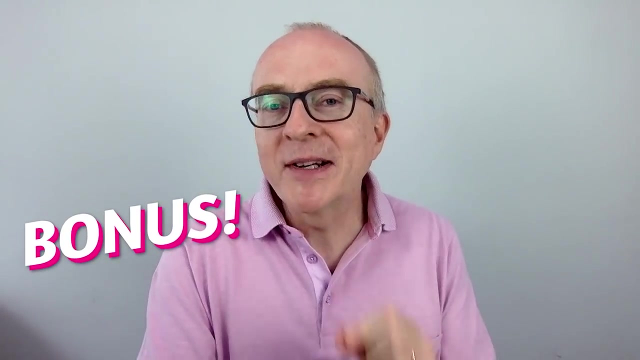 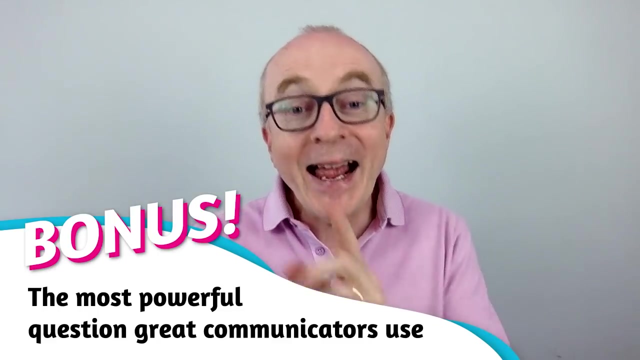 Emphasis, How to use stress effectively, Speaking clearly, Simplicity, Body language, Communicating ideas and copying others. Oh, and I've got a great bonus for you. I'm going to tell you at the end, the most powerful question that all great communicators use, And this is a really 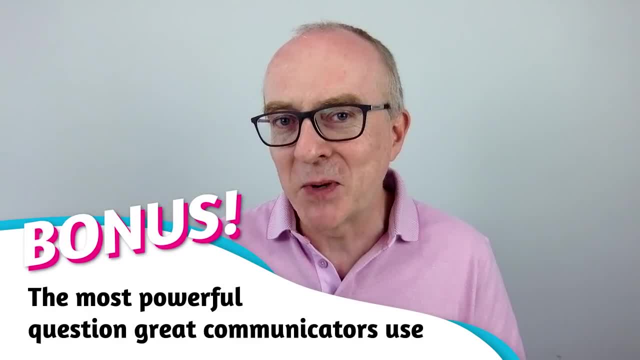 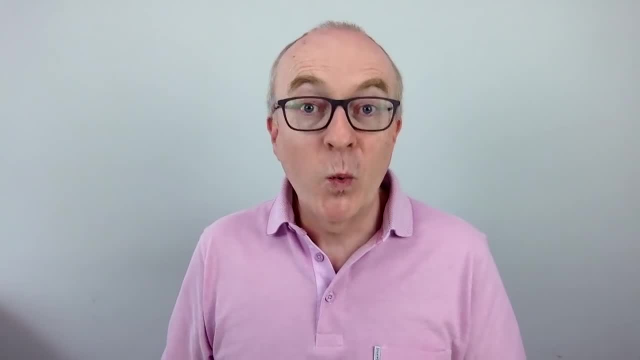 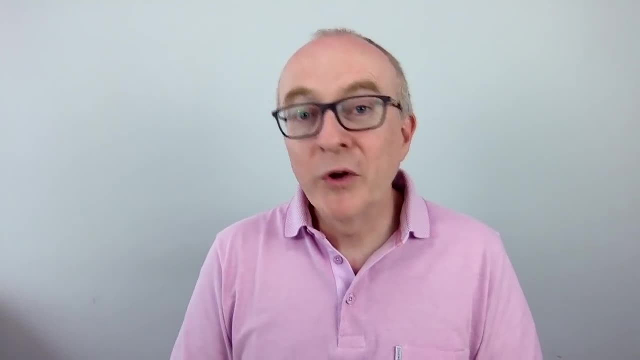 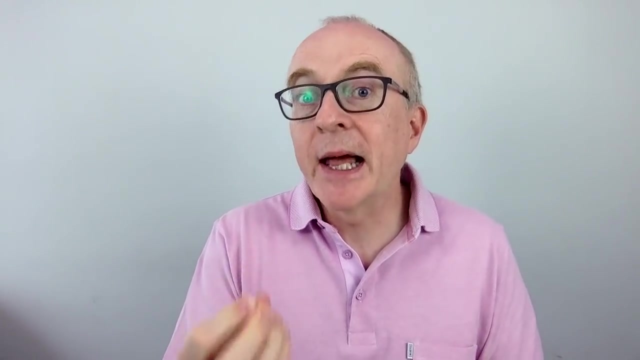 effective question you can use in the IELTS speaking test as well. So watch out for that at the end of the video. Let's get straight in with tip number one. Tip number one: Speed. Don't speak too fast. Great communicators usually speak slightly more slowly. 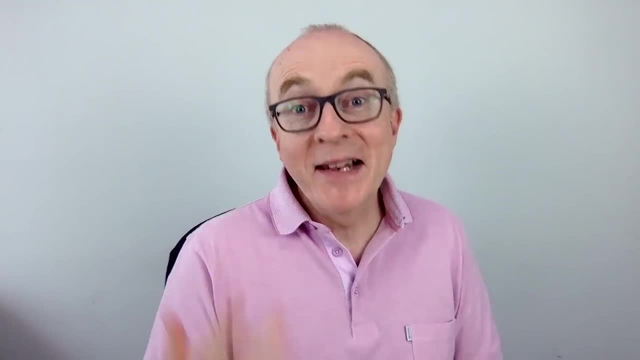 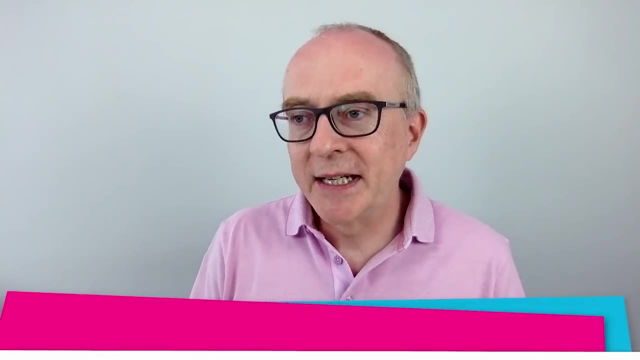 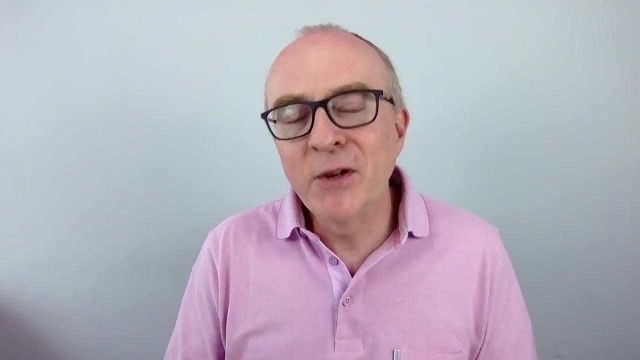 than the normal speed of a conversation, So that the listener will grasp the main idea and understand what they're saying. A problem for many students, especially if you speak quickly, even in your mother tongue, is that you think that's fluency. Speed and fluency are not the same. 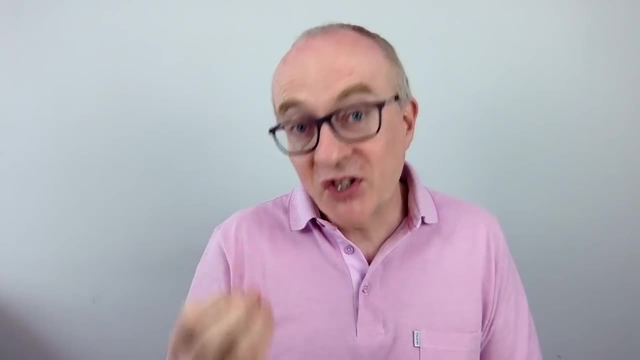 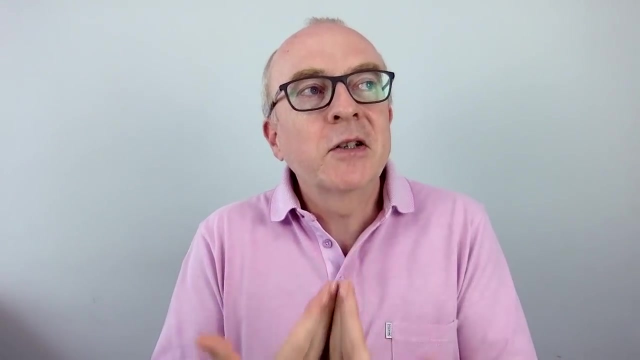 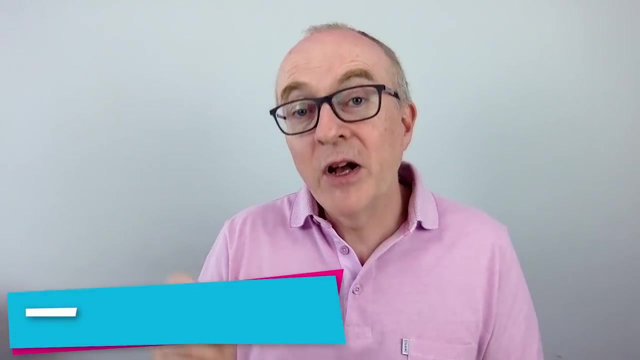 In fact, speaking too quickly is a sign that your pronunciation is not good, that you don't control the pronunciation. So when you're speaking, speak slightly more slowly than natural conversation speed And use the power of pausing. You should be pausing before you speak and in the middle of. 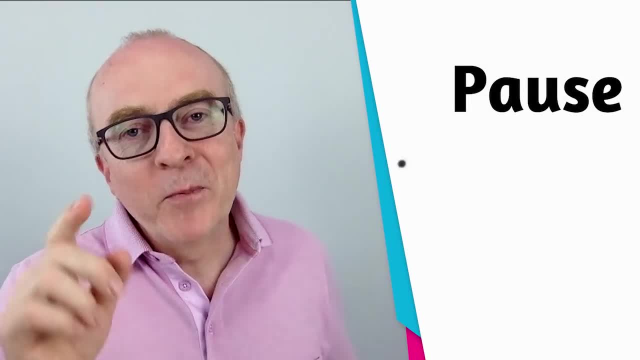 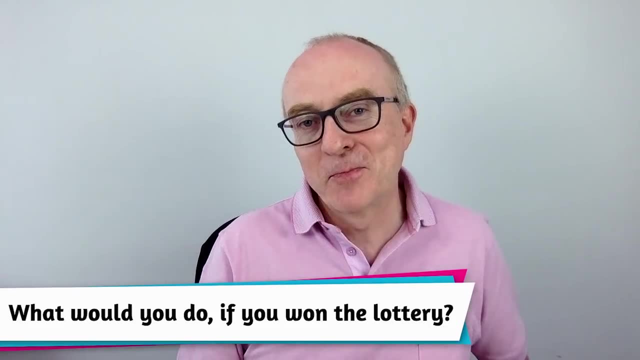 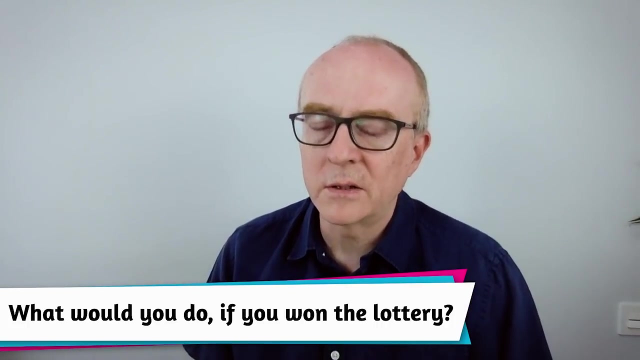 your speech, right? Let's take, for example, if I asked you the question what would you do if you won the lottery? You might answer like this: If I had a lot of money, I would purchase a majestic mansion on the rocky coastlines of Spain, Right, but now let's try and improve that. We could say: 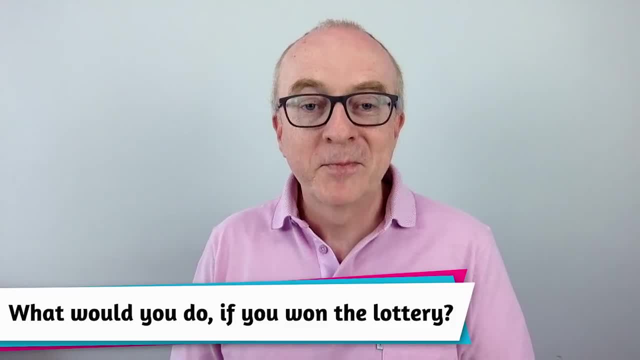 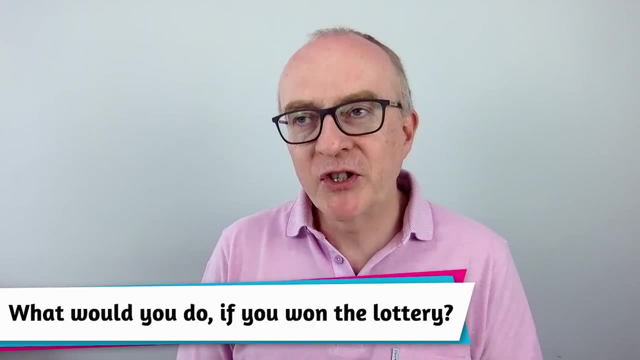 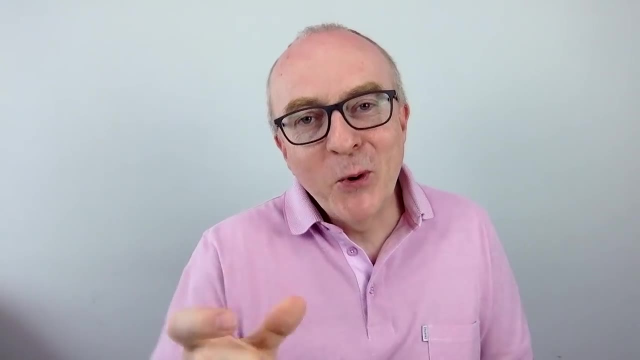 what would you do if you won the lottery? If I had a lot of money, I would purchase a majestic mansion on the rocky coastlines of Spain. Right Now, the pause at the beginning, even for two or three seconds, is very powerful. 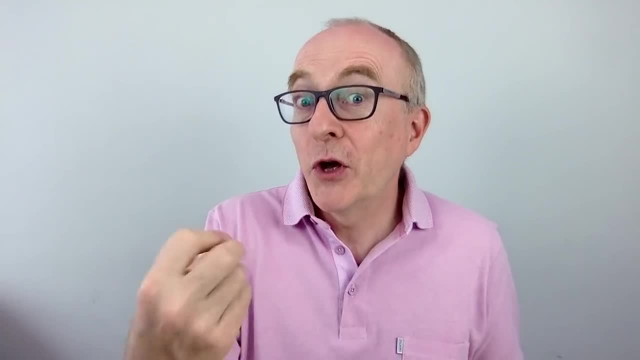 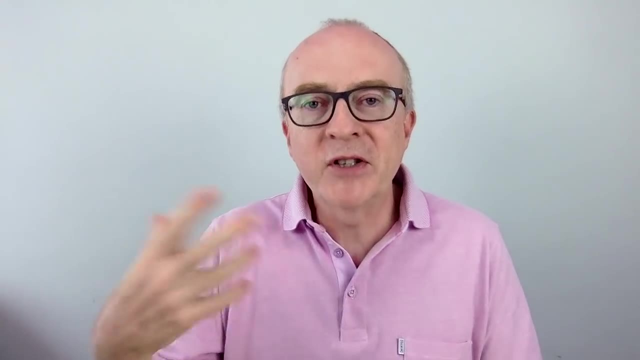 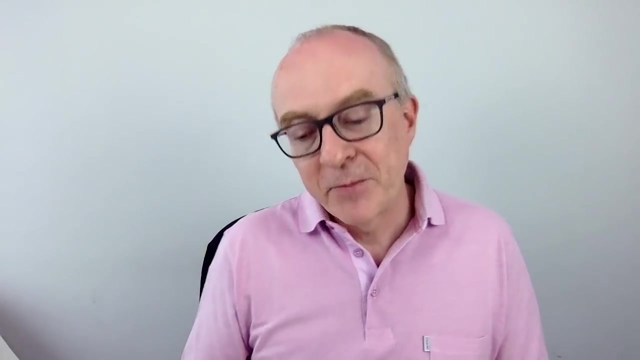 because it tells the listener that you've heard them and that you're paying attention right. It helps build trust and respect with the listener, whether it's a colleague, a friend or an examiner. So that pause at the start is powerful. And then phrasing. The phrasing is where you have a chunk and a pause in the right. 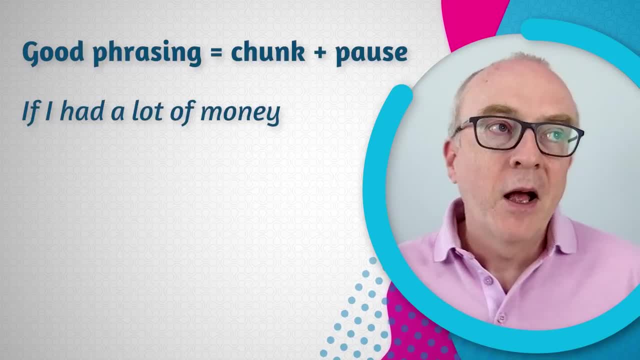 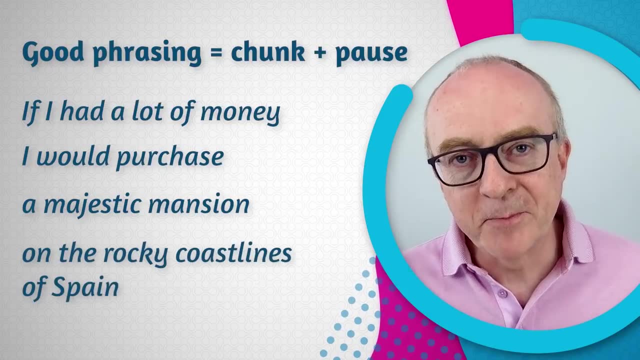 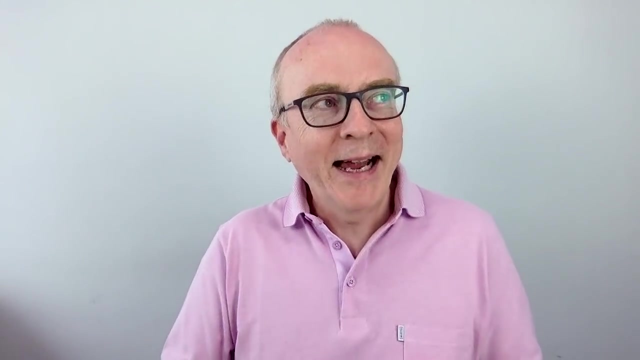 place. If I had a lot of money pause, I would purchase small pause, a majestic mansion pause on the rocky coastlines of Spain. Powerful use of pausing, In fact. I just remembered I've got a whole course about this: how to use phrasing correctly. Go and check it out. 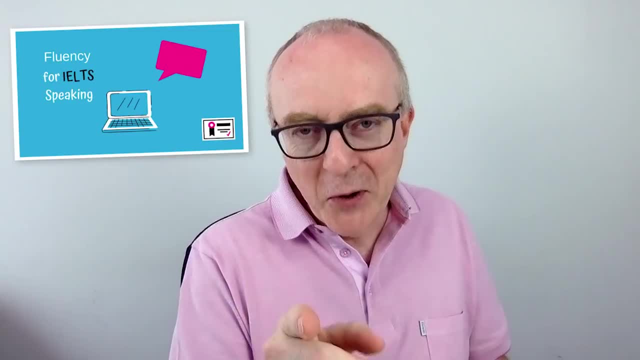 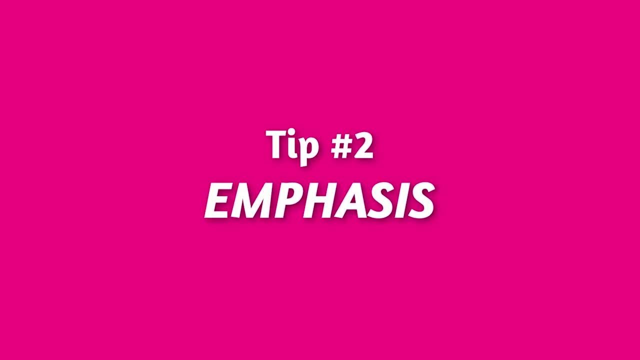 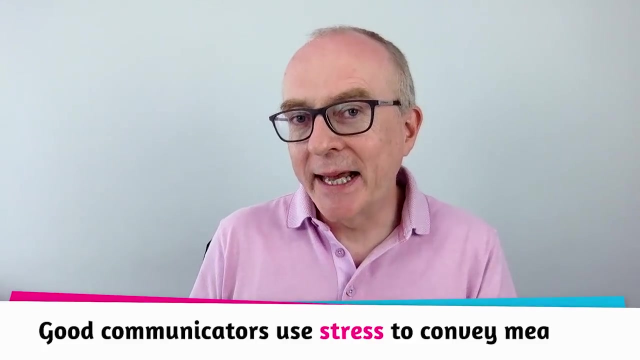 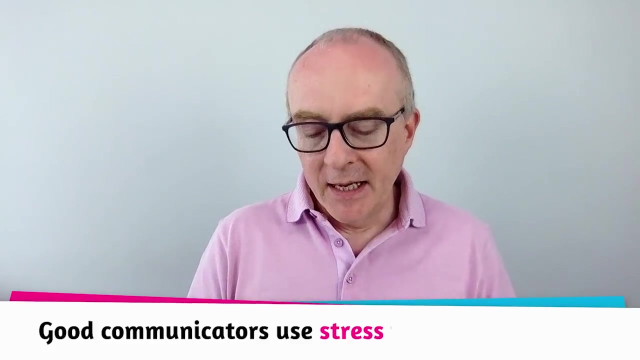 Fluency for IELTS speaking. Don't go now, go later. Right now, let's move on to tip number two. Tip number two: emphasis or stress. right, Good communicators are really good at using stress or emphasis to convey clear meaning. You need to think about stressing the right words. 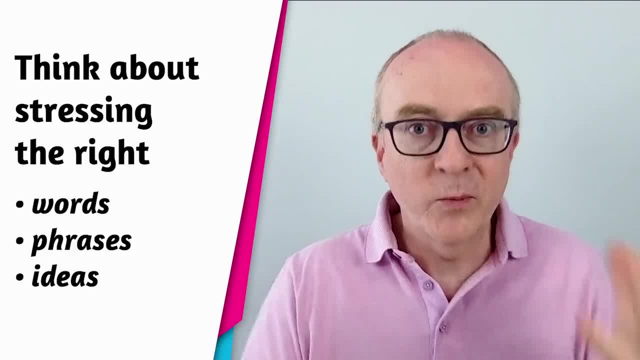 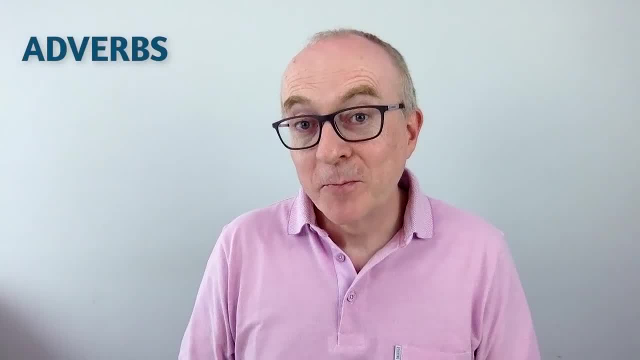 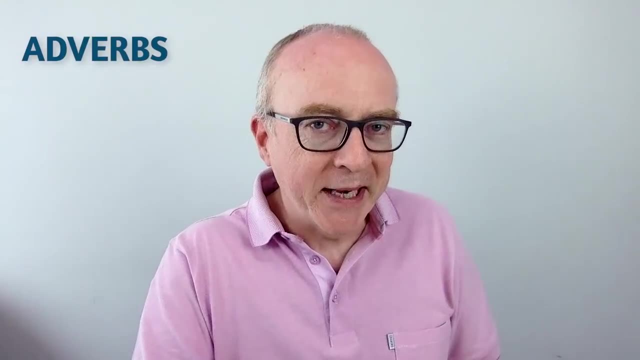 the right phrases and even the right ideas within a speech right Now. let's do this in different ways. One of the most common ways is to use adverbs. Adverbs can really help you emphasise the meaning of something. Let's take that sentence from the. 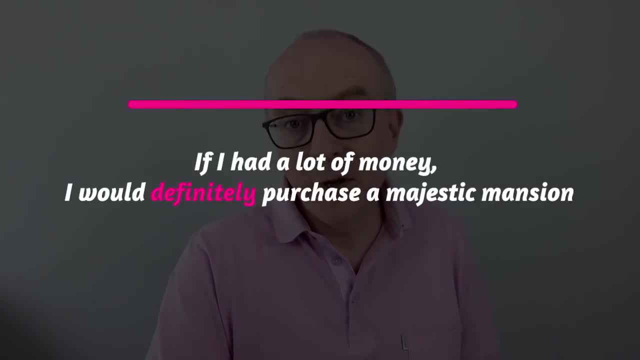 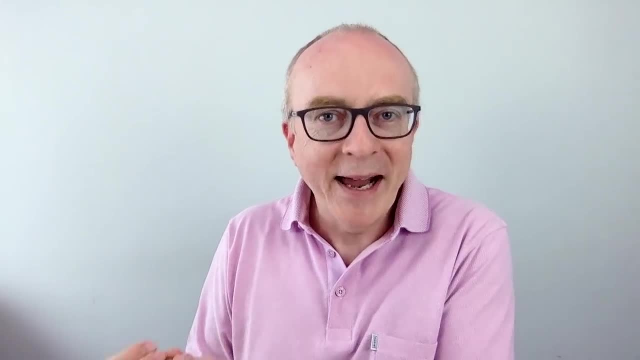 beginning right. If I had a lot of money, I would definitely purchase a majestic mansion, Definitely right. You're conveying the meaning of without doubt. for sure, that's what I would buy, right? It's a nice way to do it. 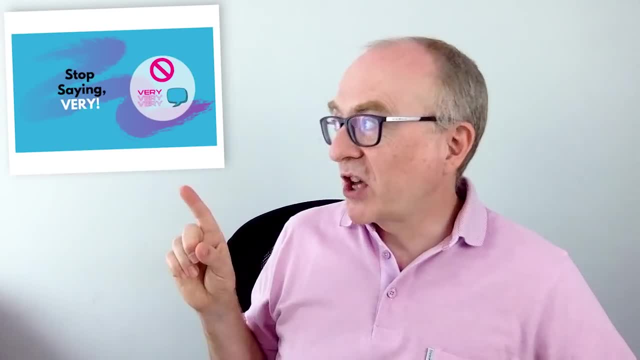 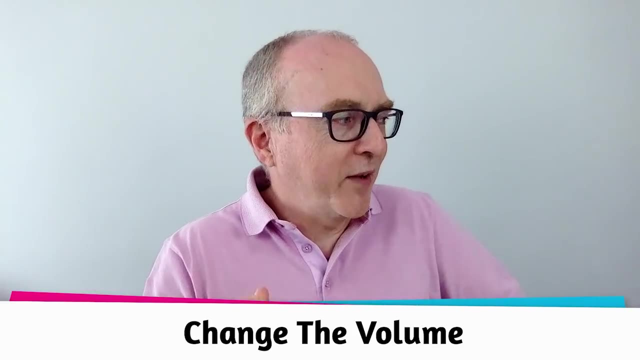 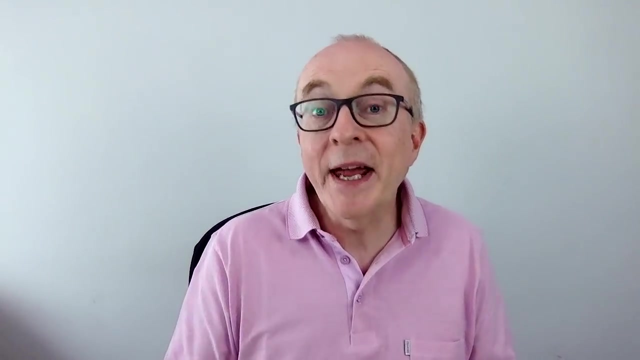 In fact, I've got a video about how to use adverbs effectively. Go and check it out later. The second thing to do is to change the volume. I'm sure if you've been to see some live music right, You'll notice how in music they use volume- changes in volume- to convey meaning. 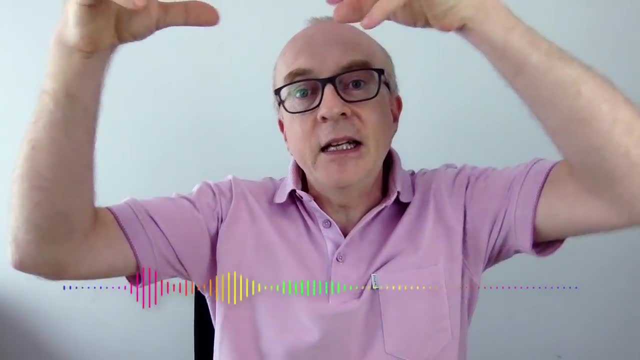 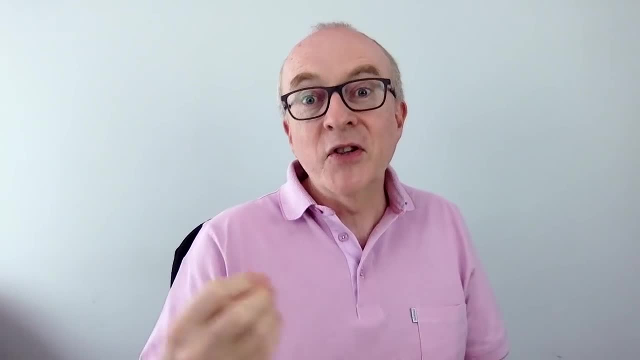 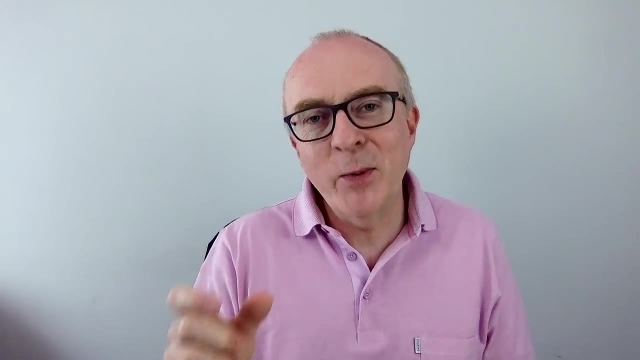 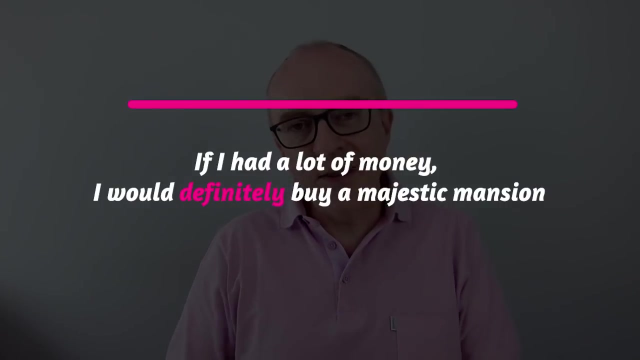 You're speaking right. You go from being very quiet to then getting louder and it changes the dynamics, particularly with adverbs. If you're stressing, when you stress something, you can increase the volume right. If I had a lot of money, I would definitely buy a majestic mansion. 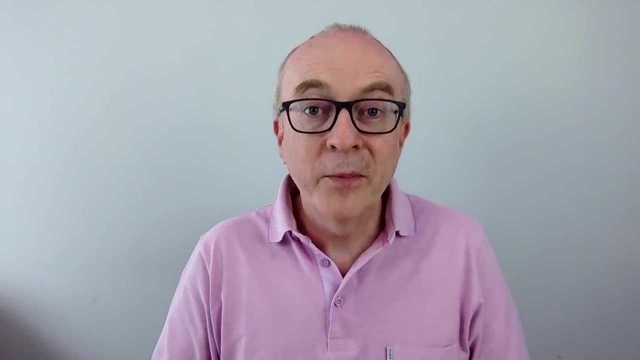 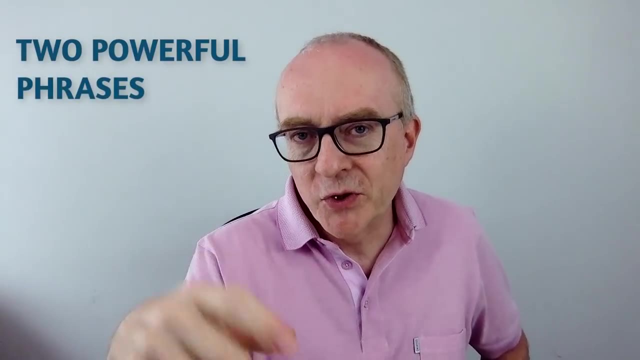 That volume change. really good to help with that. Now, another couple of things. There are some things that I like to do And if you were here, I'd definitely buy a majestic mansion. some very useful phrases you can use to help you show emphasis and stress. 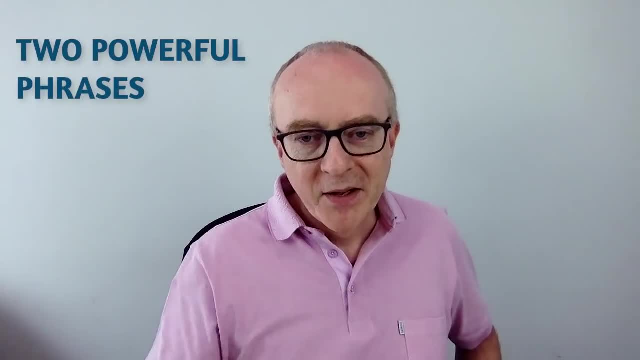 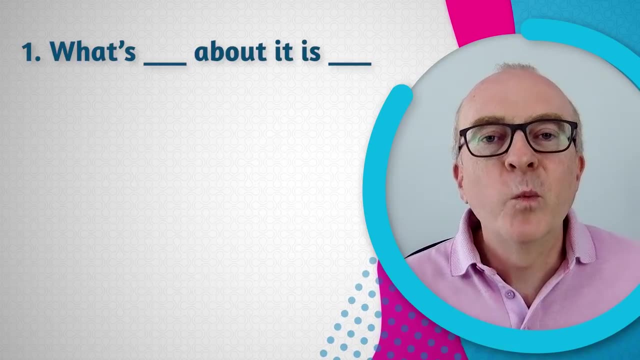 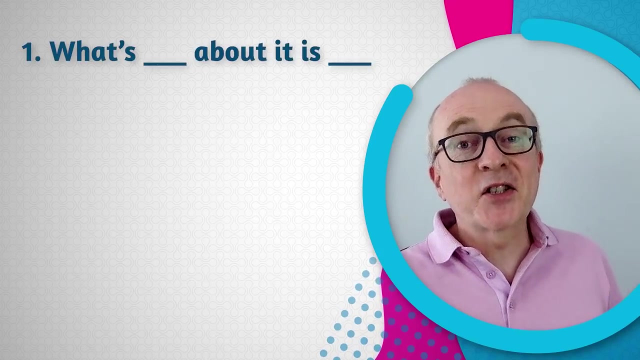 and communicate more clearly. The first one is this one: What's blah blah blah about it? is this right? What's interesting about it is, or what's amazing about it is. So if somebody asks me, for example, is Spain an interesting place to live? 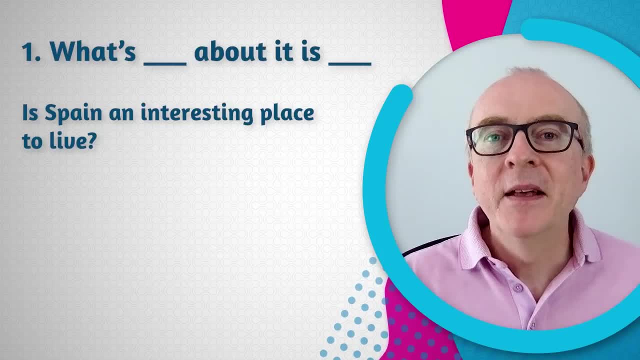 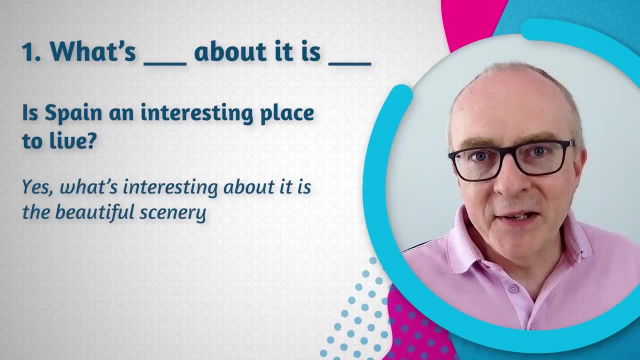 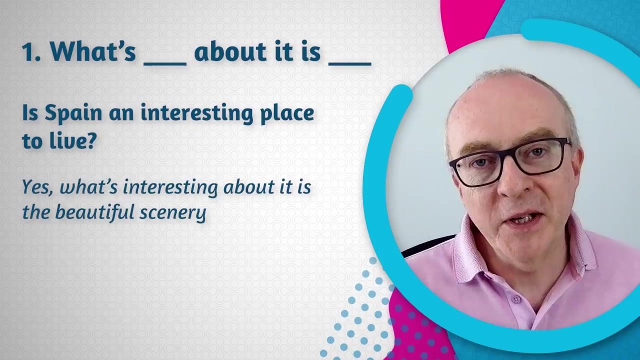 I can say, well, yes, it's interesting, Or yes, what's interesting about it is the beautiful scenery. How much more powerful is that? right, We're focusing the attention. What's interesting about it is: it's a lovely way of doing it. 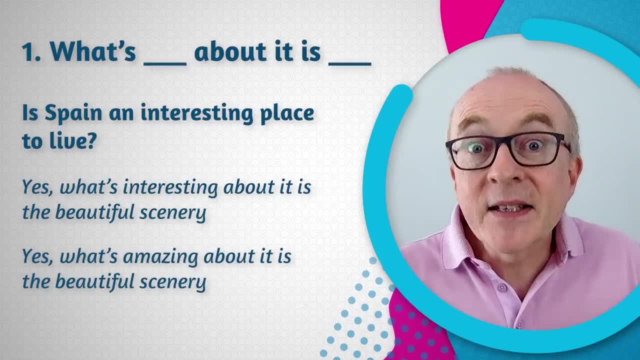 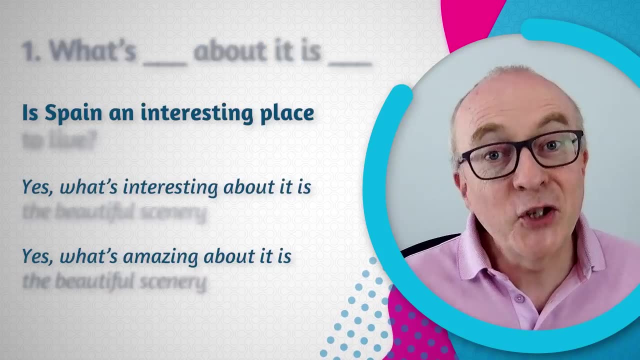 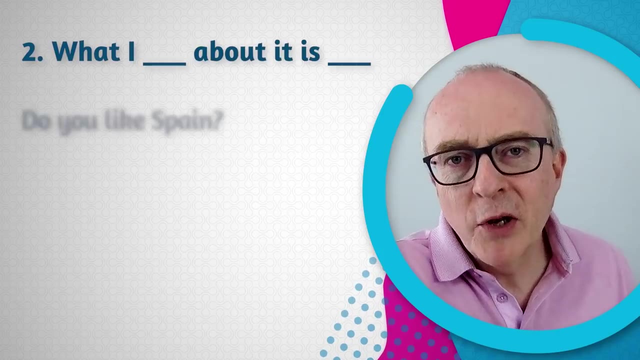 What's amazing about it, what's fascinating about it? you can have different adjectives in there. Similarly, another phrase you can use is: what I blank about it is. so again, if somebody asks me: do you like Spain? Yes, I do, I like it. 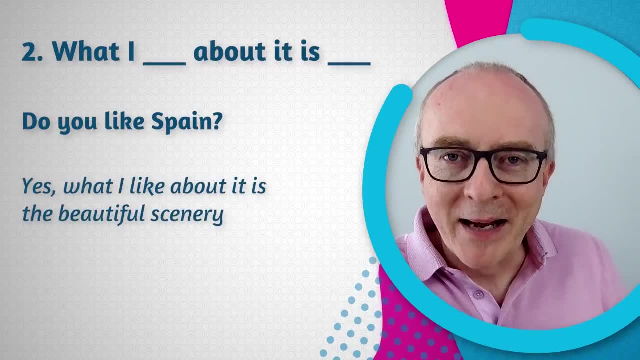 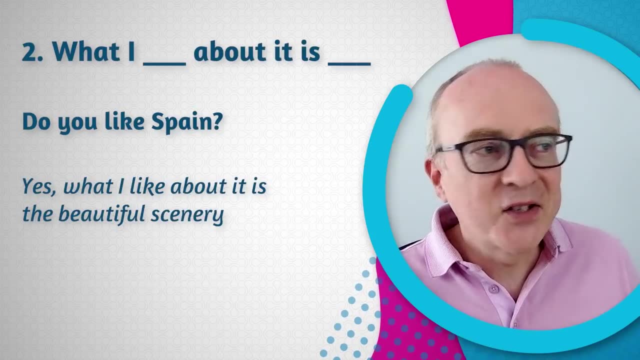 Or yes, I do. What I like about it is the beautiful scenery. You see the stress. What I like about it is da da, da, da, da Again, you can change verbs. What I hate about it: 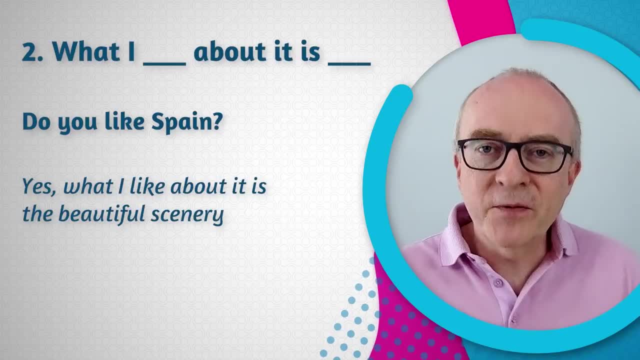 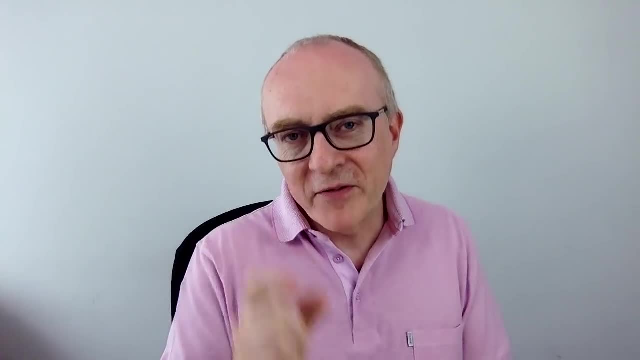 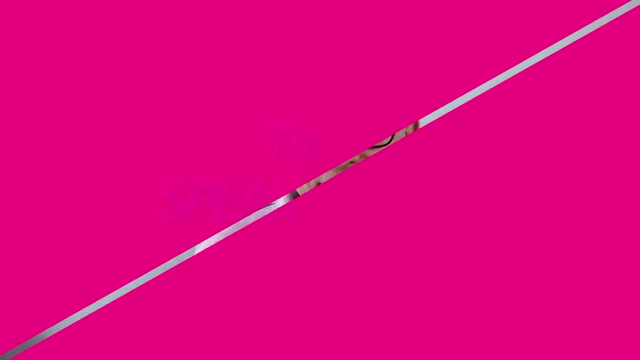 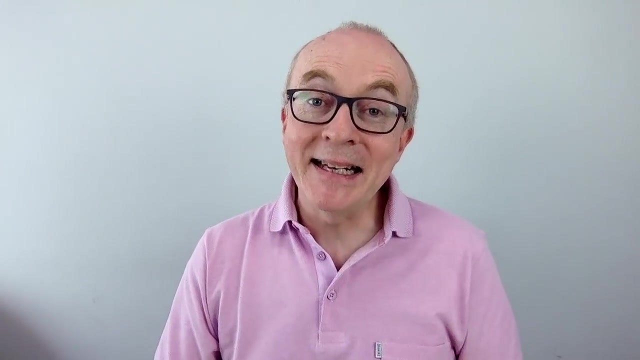 what I love about it is nice focus, lovely way to emphasise and stress the meaning you want. So two great phrases there that you could use to help convey your meaning and be a better communicator. Let's move on. Tip number three is speak clearly. 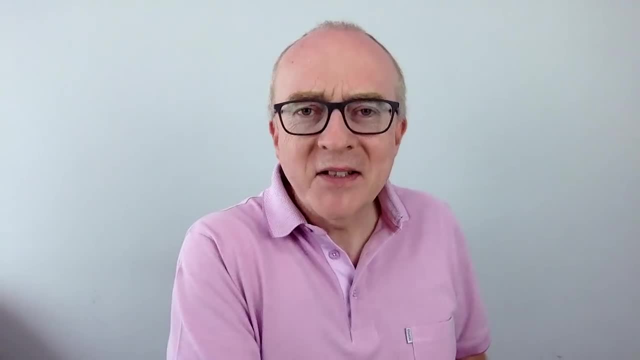 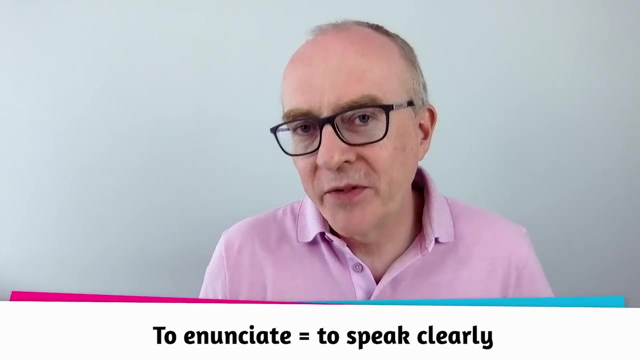 You really need to enunciate. Ooh, there's a nice word. enunciate, It just means to speak clearly, open your mouth. English is one of those languages where a lot of the sounds come from the front of the mouth. 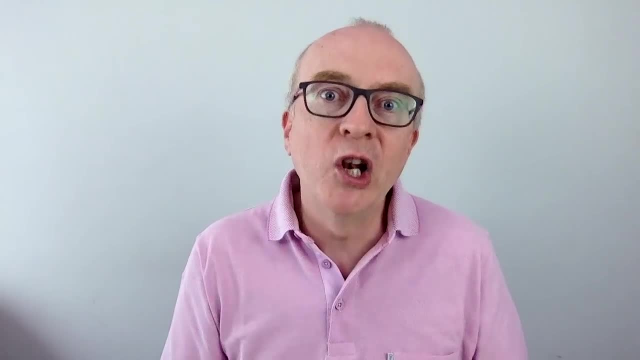 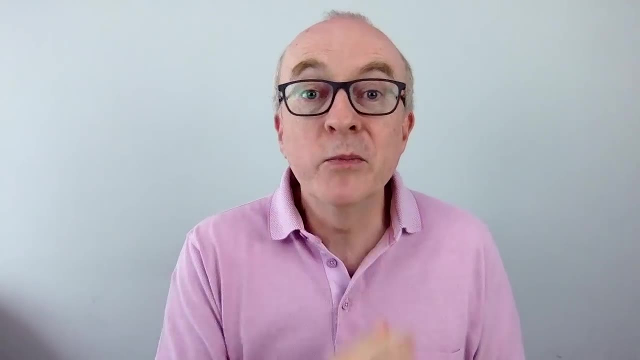 We use our lips and the shape and the jaw a lot, a lot more than some languages. right, In some languages you can see people speak almost without moving the lips. Hello, my name is Keith. Nice to see you. How are you? 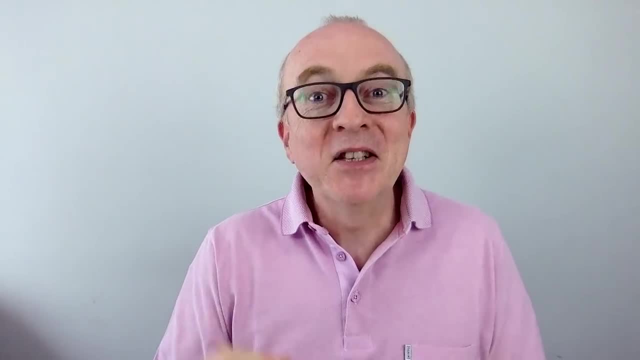 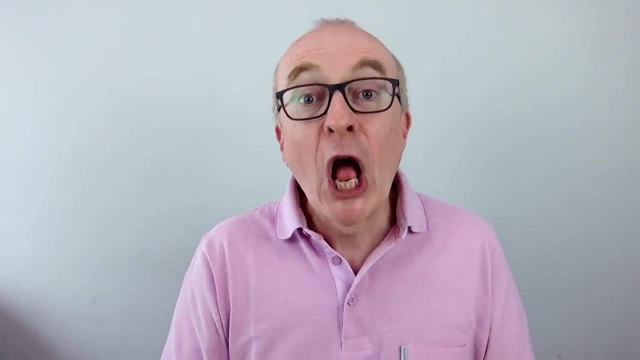 Things are good, thank you. What you need to be practising is to over-exaggerate. Practise almost like a muscle gym, like a mouth gym, Oh, oh, oh. Practise moving your lips. So a very good exercise is to look in front of a mirror. 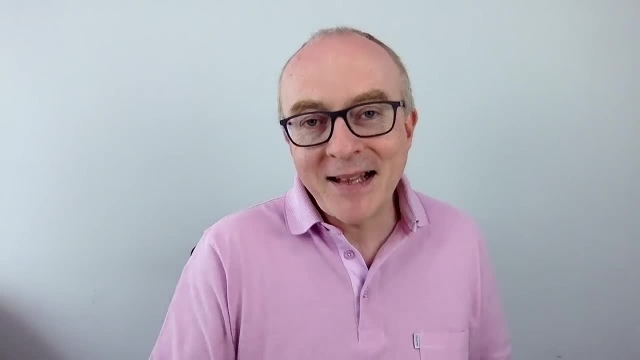 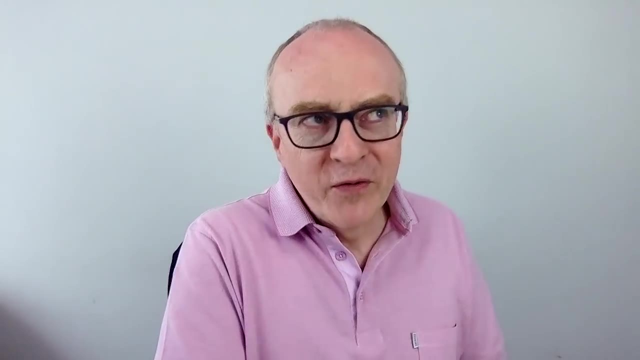 as you're speaking and over-exaggerate the movement. Let's take that sentence that we've been using in this video and just watch my lips right As I over-exaggerate. If I had a lot of money, I would purchase a majestic mansion. 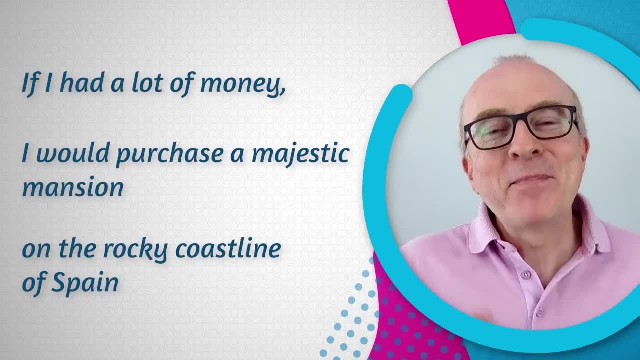 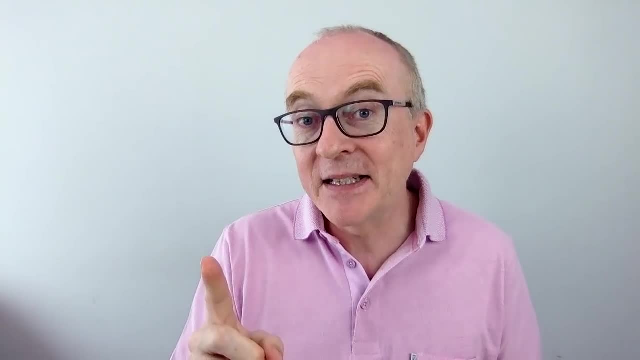 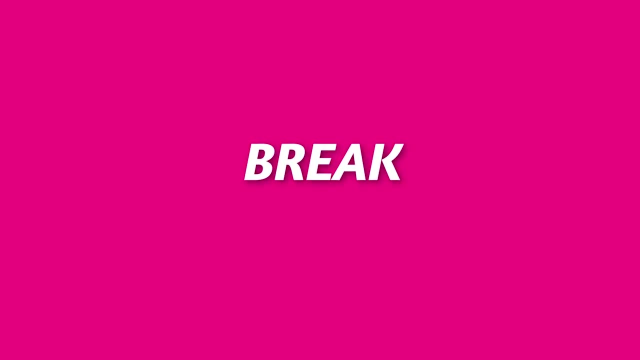 on the rocky coastlines of Spain. And that's it Now you over-exaggerate. When you're in conversation, you just speak, naturally, But when you're practising, go a bit over the top. Let's move on Now. I'm ever so thirsty. 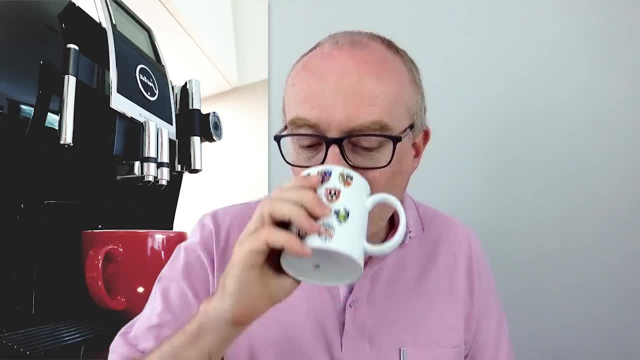 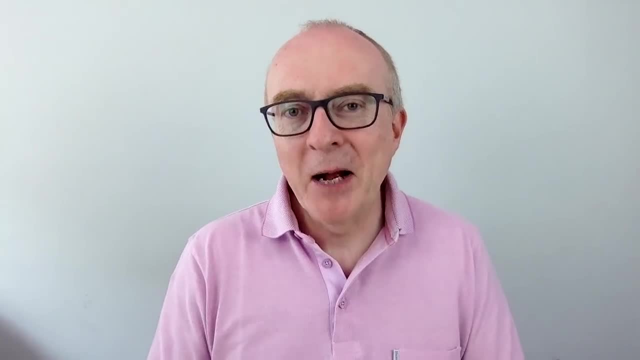 Let's have a drink. What would you like? Hmm, Excellent, good Listen, I hope you're enjoying the video so far. If you are, then do subscribe and turn on your notifications. If you are, then do subscribe and turn on notifications for future videos. 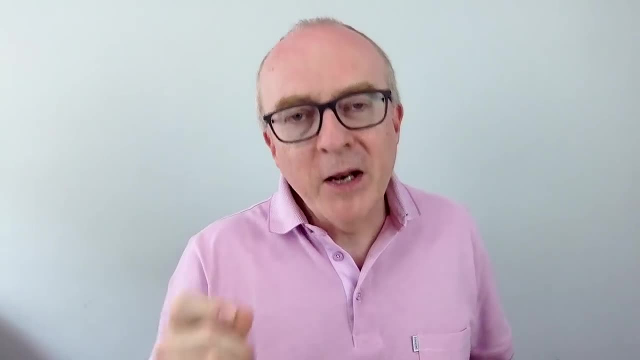 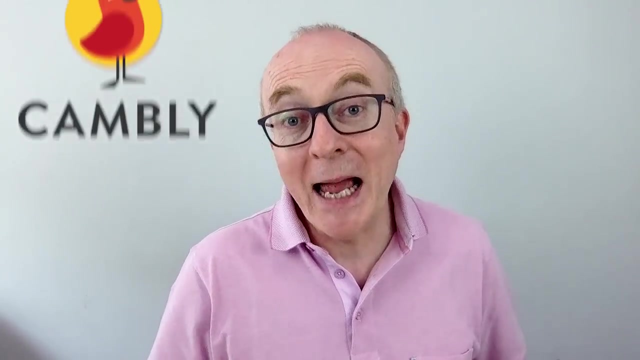 I'd just like to take a moment to tell you about developing your communication skills, right? In order to do that, you need to practise, And a great place to practise is on Cambly. Cambly is an online platform with native English-speaking teachers. 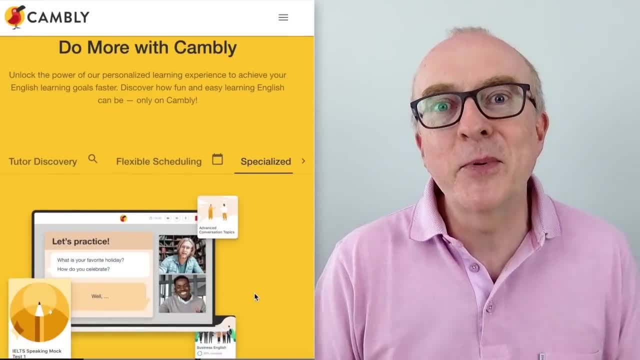 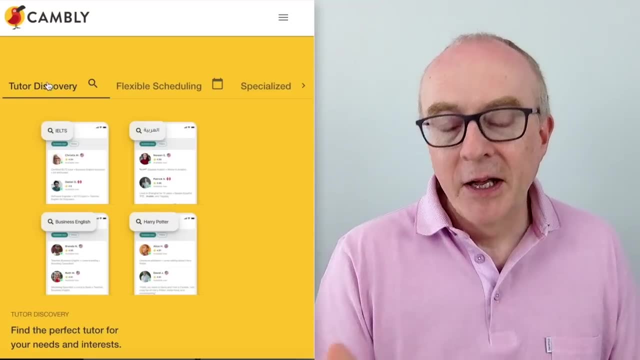 where you can have one-to-one classes with teachers and develop your speaking and communication skills. It's great because you can choose which teacher you'd like to have You study when it suits you and you even decide what you want to do in the class. 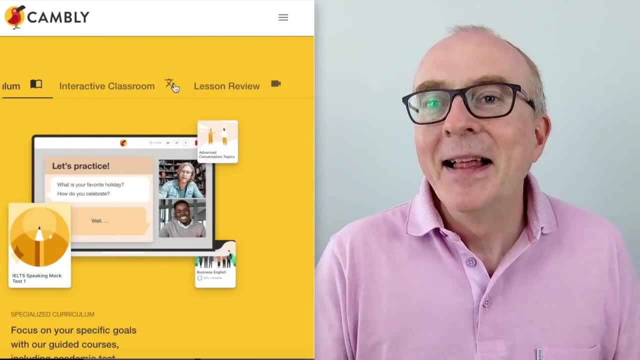 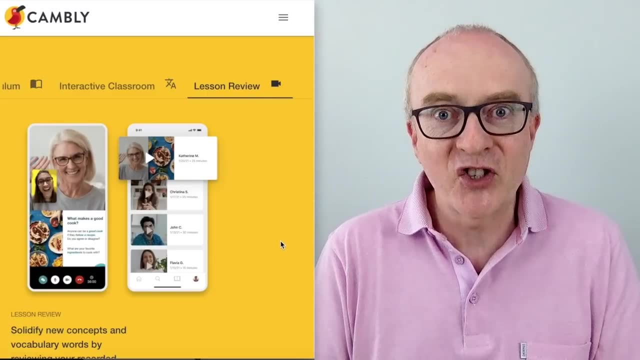 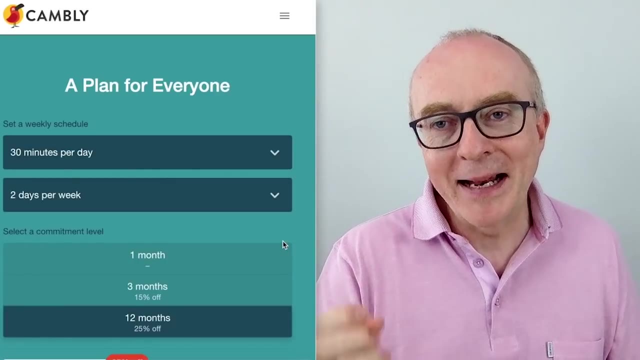 or your teacher can guide you if you like. It's great because you can also record the classes and then go back later to watch again and carry on practising and studying. Cambly have a variety of different plans for different needs, and I'm sure you can find a plan that will suit you. 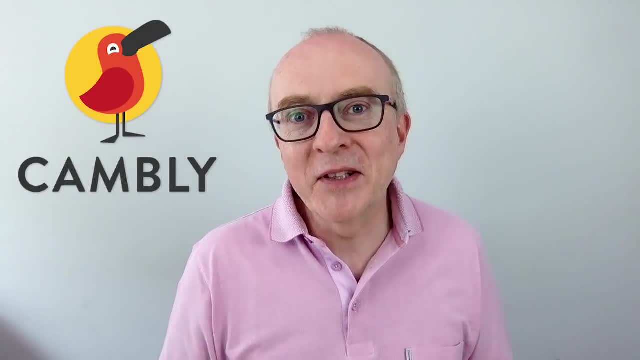 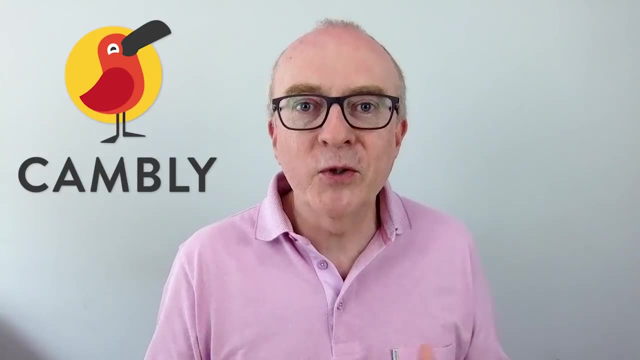 As you are one of my students and as Cambly are sponsoring this video- thank you so much, Cambly Camberley, for that- then we've got some discounts for you. If you are a first-time user, you can get. 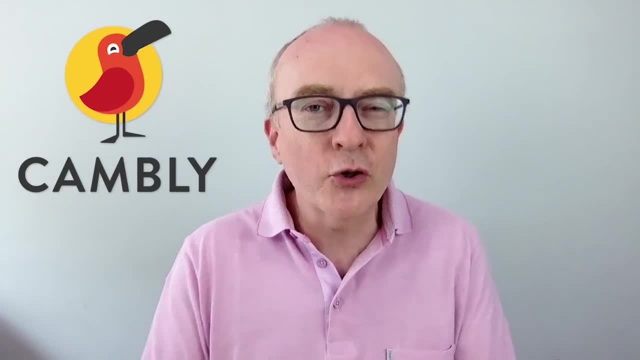 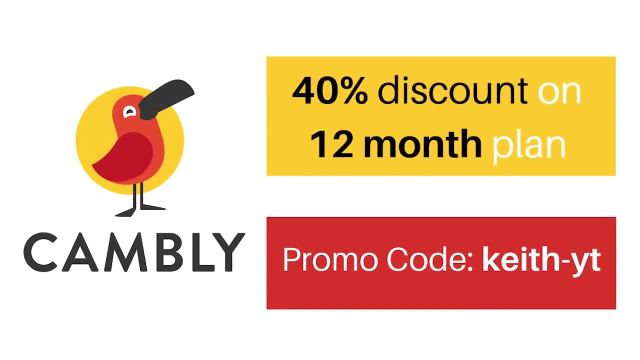 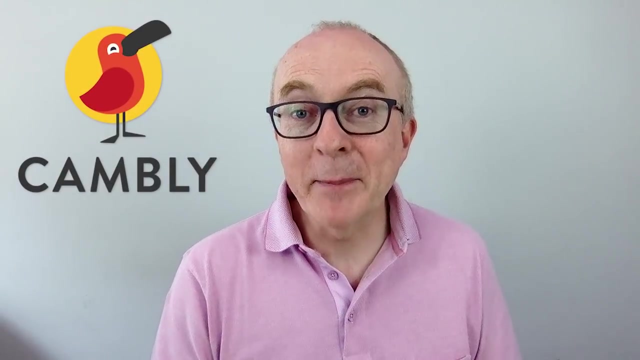 a 10-minute class for free, just to practice and try out the platform to see if you like it. If you go for the one-year plan, that's 12 months- you get a 40% discount off the regular price- Great saving. If you sign up for Camberley, remember to use the code KEITH-YT to get your. 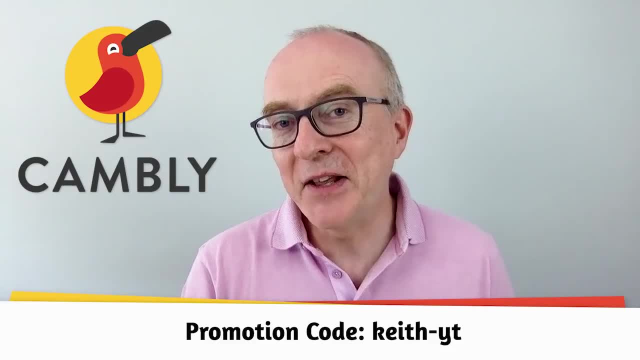 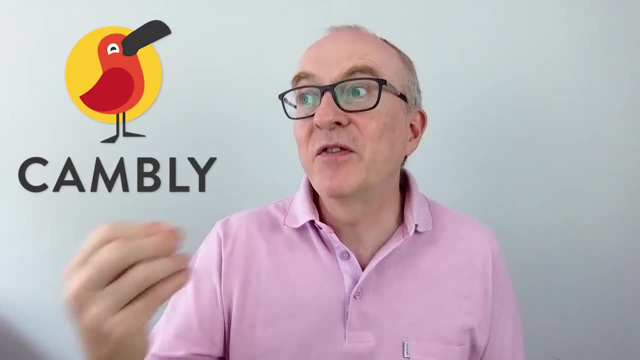 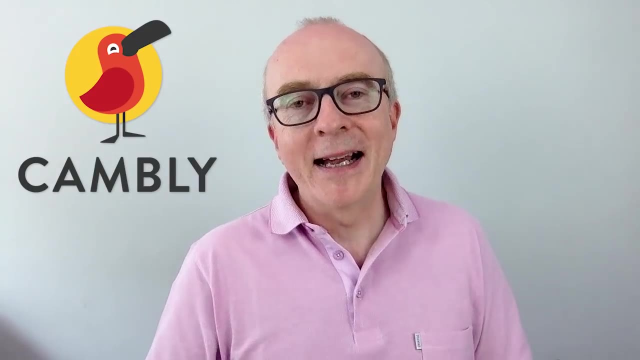 40% discount on the 12-month plan. That's KEITH-YT. I think preparing for IELTS is all about improving your English for the long term- right English for life. It's worth investing in a long term plan- 12 months- and improve your English. Go and see. You can check out the links below. 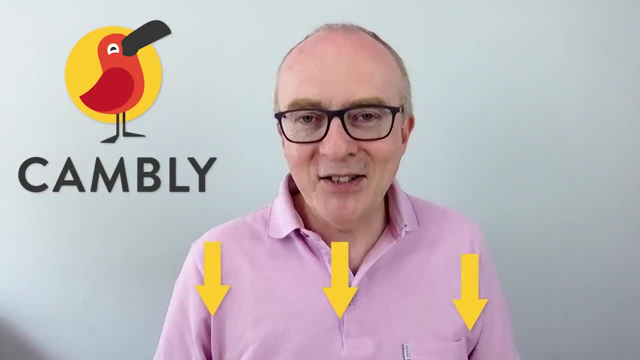 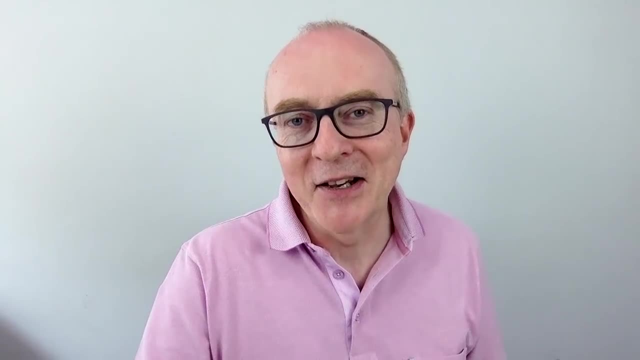 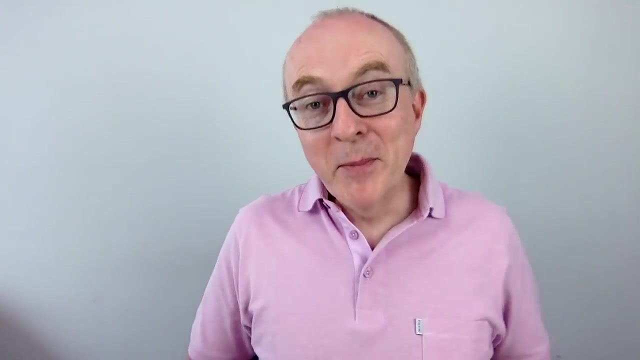 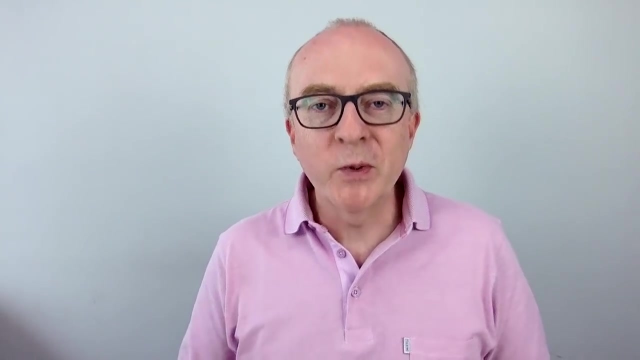 to go and check out more, See if it's right for you. Excellent. Now let's get back into those tips to help you. Tip number four: simplicity, or keeping things simple. Did you know there's a huge difference between spoken English and written English? I've talked a lot about this, but if you don't believe, 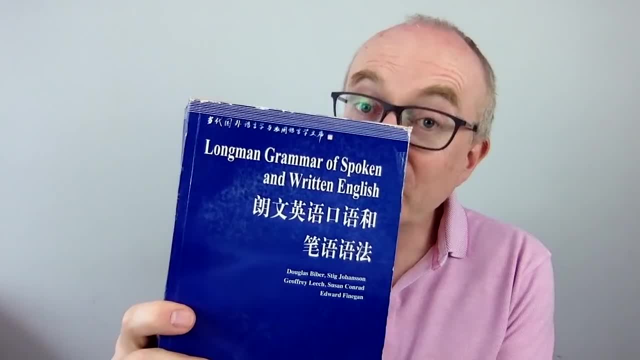 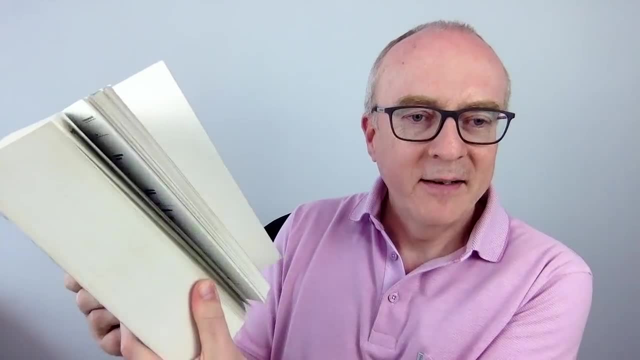 me take a book like this, right Longman Grammar of Spoken and Written English. I got this in China, but it's the British. I mean, look right, This is a mammoth volume. The differences, I mean it's huge. 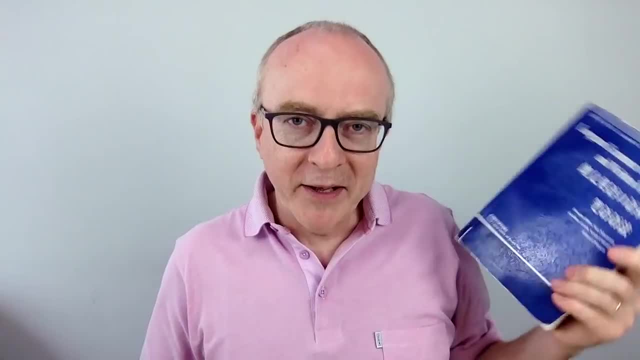 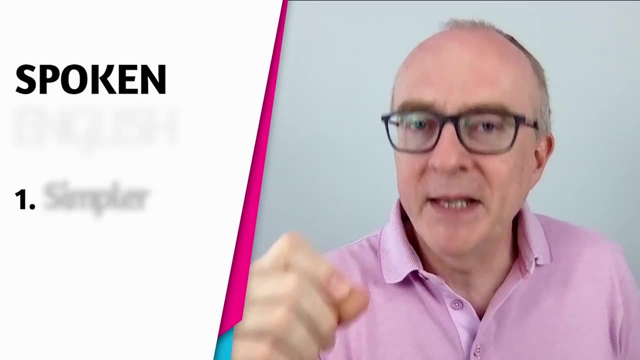 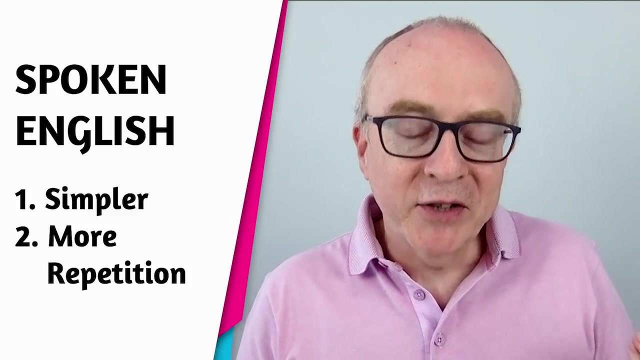 There are big differences. Let me do that Blinkist thing where I summarise this in one minute. Two of those differences is right is that spoken English is generally simpler, It uses more simple language. And the second difference is spoken English has more repetition. 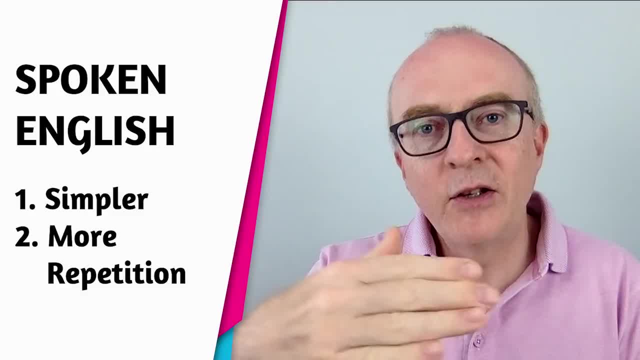 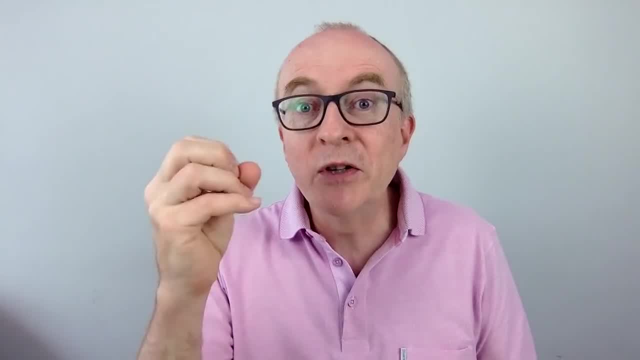 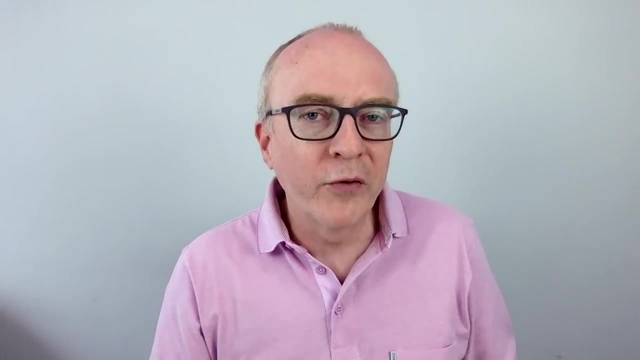 Which is logical, right, Because when you're writing, you can read things again and again. You don't need to repeat the words. When you're speaking, words disappear. People forget, So you need to repeat things again, often in a slightly different way, but a lot of repetition. 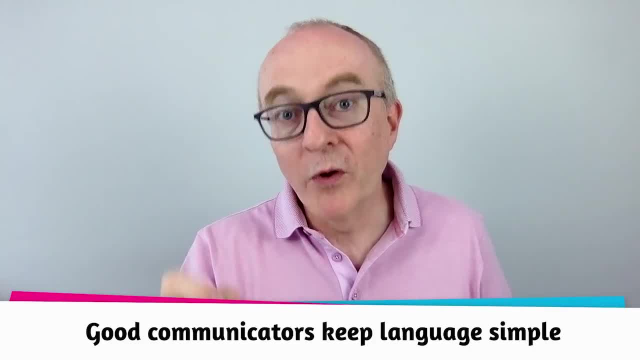 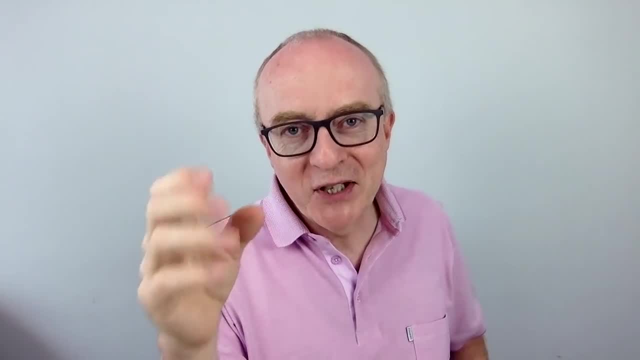 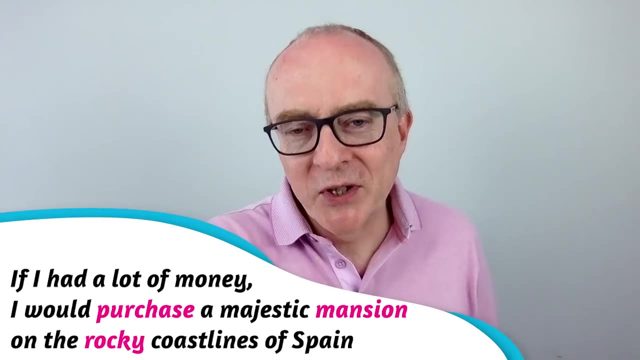 So the idea of keeping language simpler is an important one when communicating effectively. Do you remember that phrase we had at the start about purchasing the majestic mansion- this one right Now? I would ask the person who said this: okay, if I had a lot of money, that's fine. 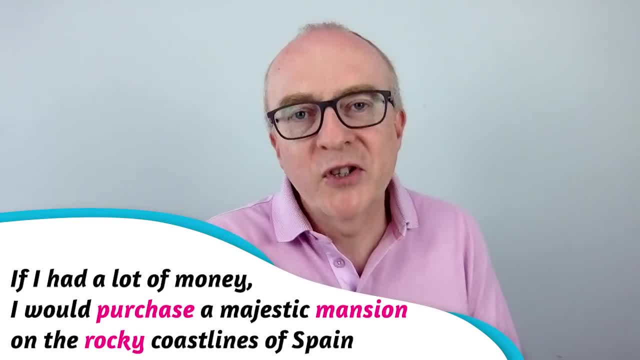 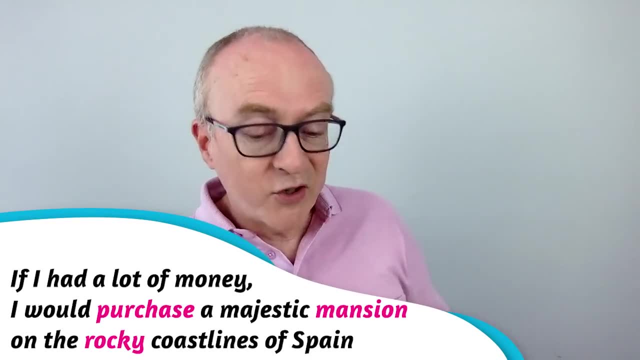 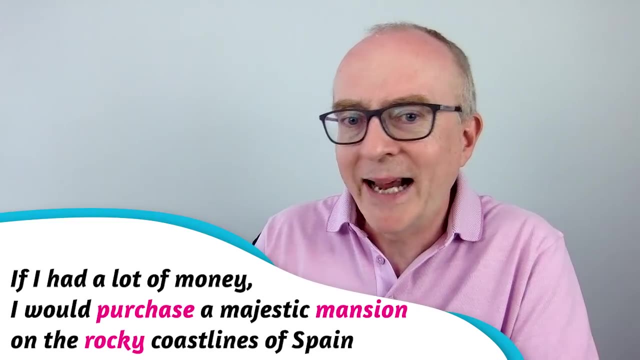 Purchase, we would probably say buy, but you could say purchase Majestic mansion. That sounds poetic. Why did you use majestic mansion? Oh no, I just looked it up in the dictionary yesterday. Right, It might be better to say well, a house or a huge house, right? 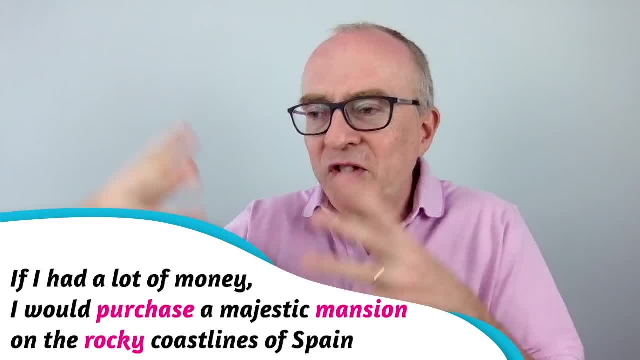 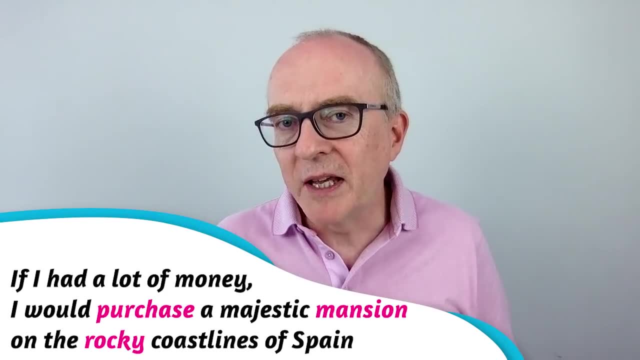 Right. It might be better to say well, a house or a huge house right, To get the meaning much clearer. It's about the size of the house. It's a huge house. Rocky coastlines. Why did you say rocky? Oh yeah, because I looked up rocky and it was a. 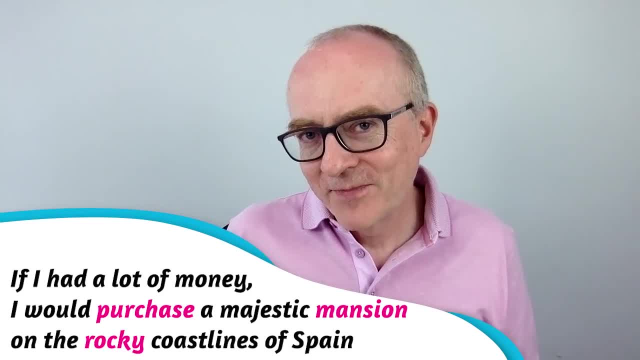 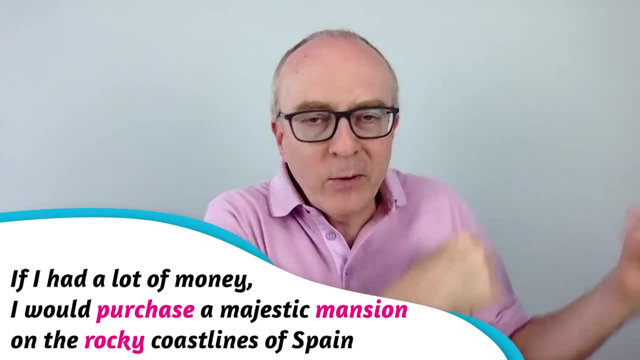 nice word to show off. Is it important? right? The fact that you're buying a house is the fact that it's rocky important? No, Then out, forget it. right On the coast of Spain, If I had a lot. 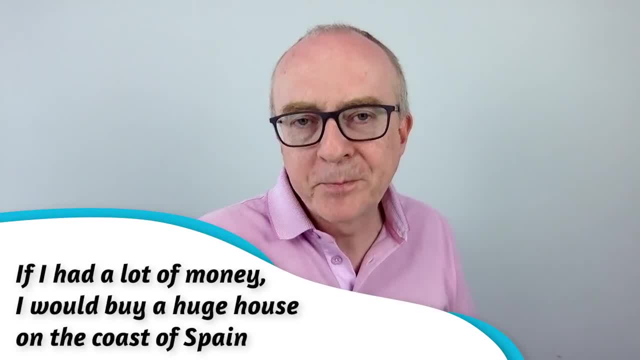 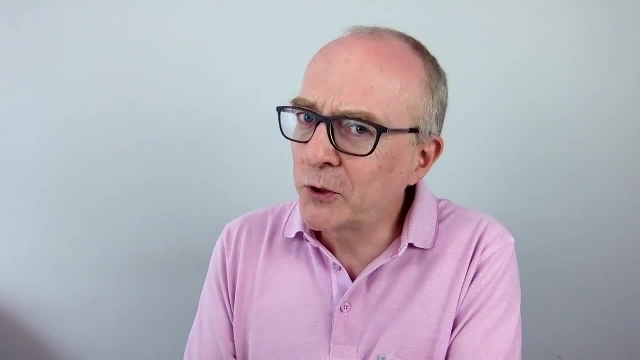 of money, I would buy a huge house On the coast of Spain. That is much more effective communication. Now I know what you're thinking. You're thinking, Keith, but in IELTS speaking we need to use complex vocabulary. 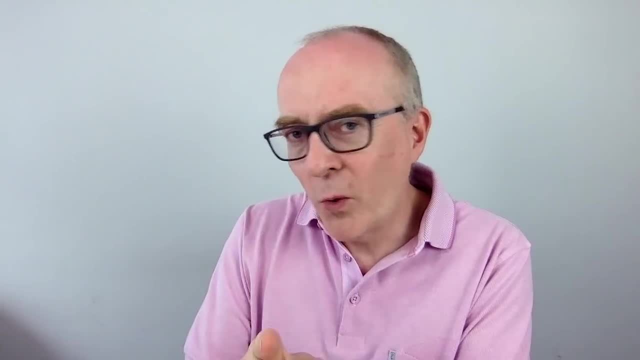 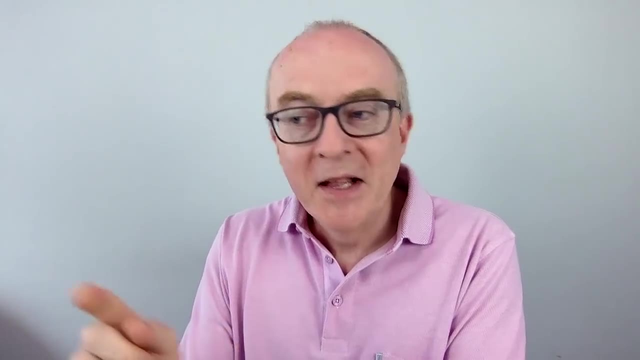 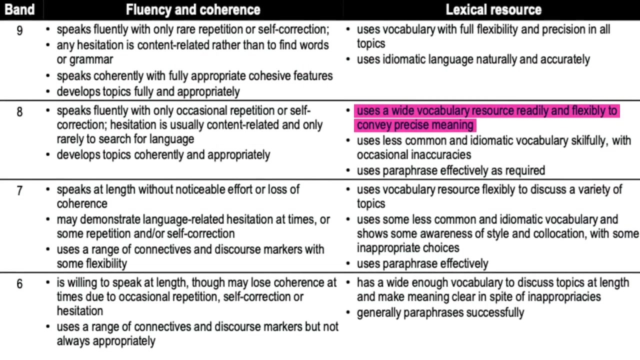 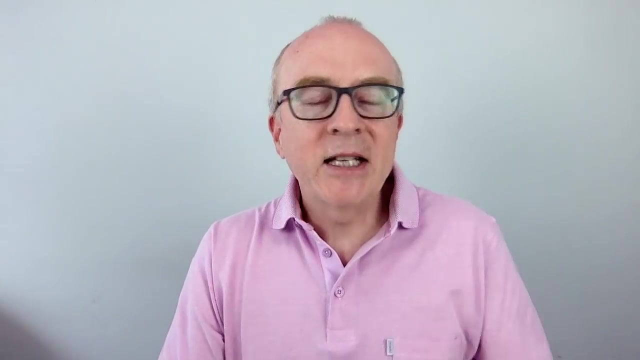 right. Yes and no. In fact, not quite at all. There's nothing in the band descriptors about complex vocabulary. The band descriptors talk about band eight. right Uses a wide vocabulary resource Readily and flexibly to convey precise meaning. Using vocabulary flexibly: It's about using the 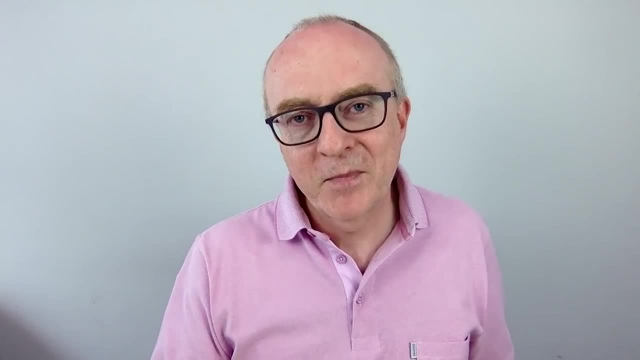 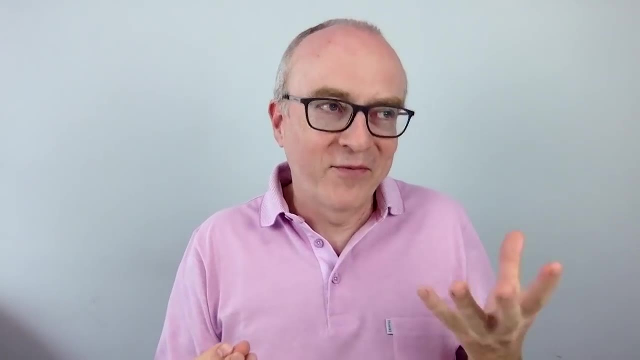 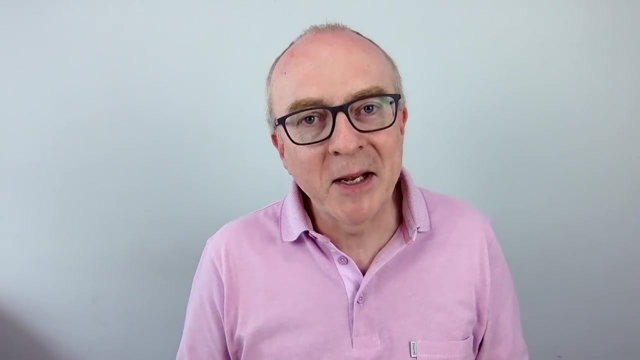 right words in the right place at the right time, Not necessarily complex. Now I do agree there's a bit of a balance between showing off vocabulary but using the right words at the right time, flexibly. So it's not always the same thing, okay, Just bear that in mind. Simplicity helps you. 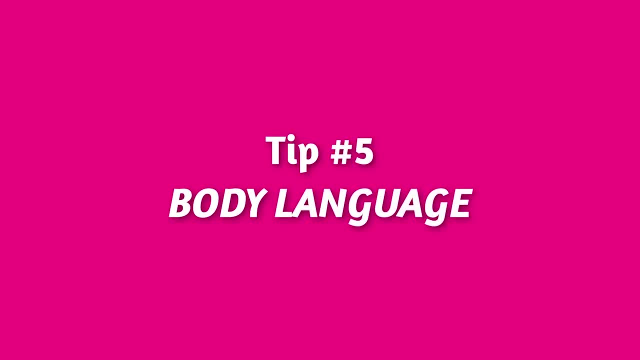 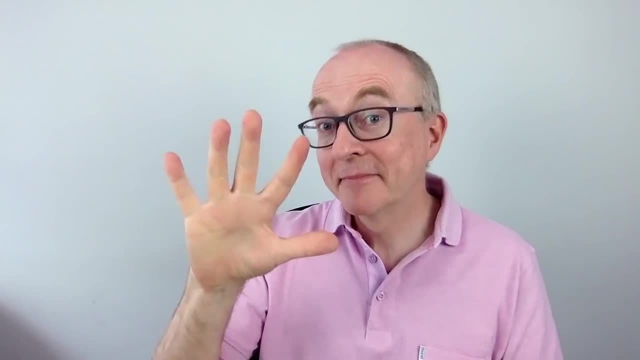 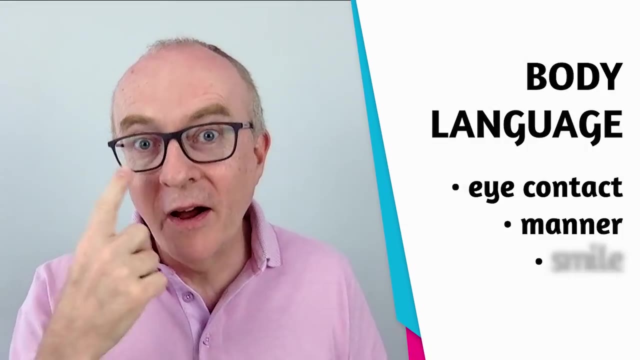 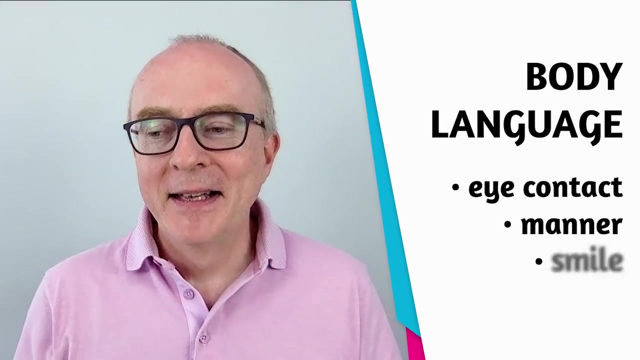 communicate. Let's move on. Okay, tip number five: Ready Body language. Now this includes eye contact, your manner- whether you're friendly or unfriendly- and smiling. Communication is far more than words. right, We communicate with words, but actually we're not talking about words. We're talking about 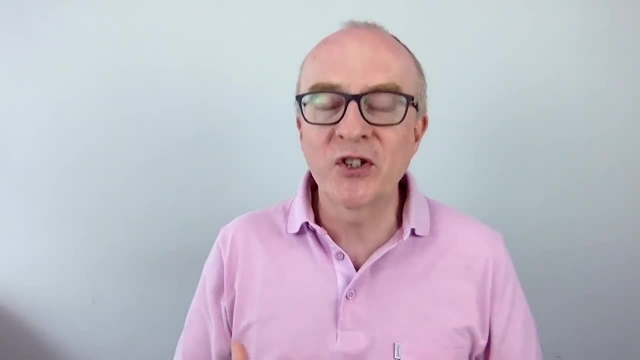 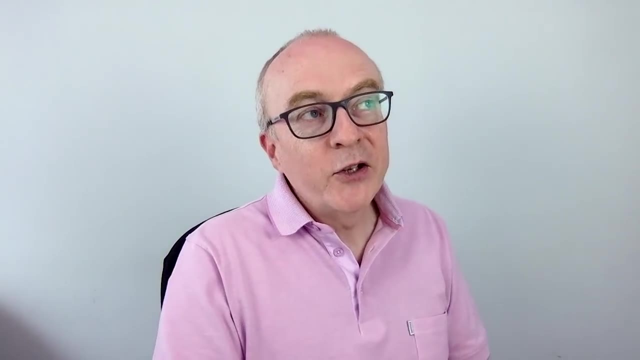 our body language. Actually, we communicate a lot without words, just through our body language, And it's very important. Take a simple example. Let me show you different ways I can use body language and words to ask for your pen right. First, 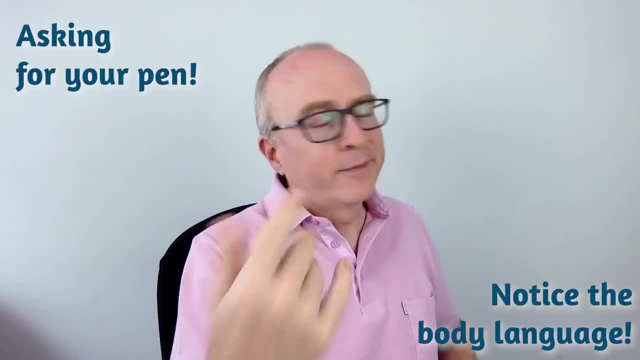 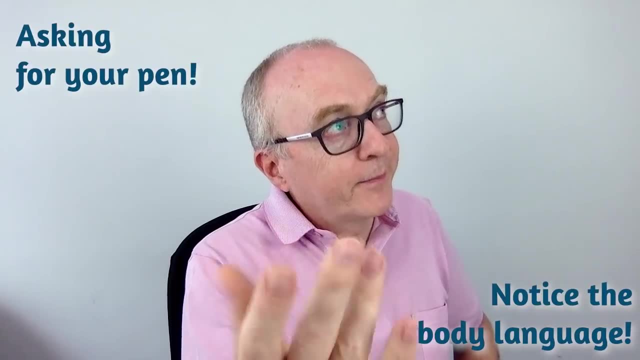 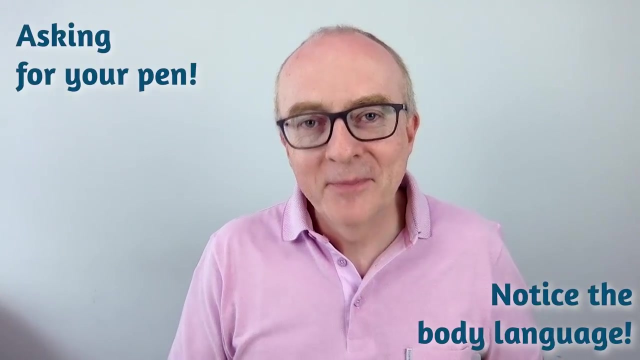 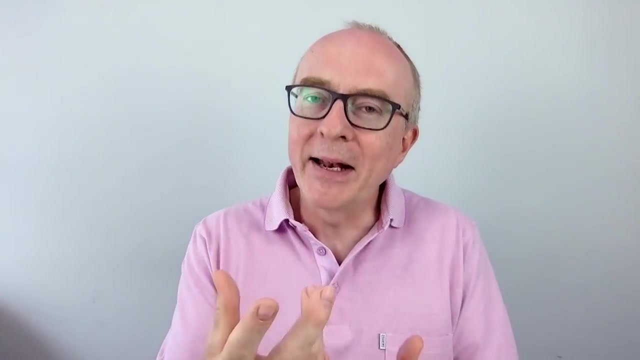 Second Pen. Third, Give me a pen. Fourth, can I borrow your pen please? Thanks, Which one is more effective? right, It's not only the words, but it's the manner, the gestures that we make as well. I. 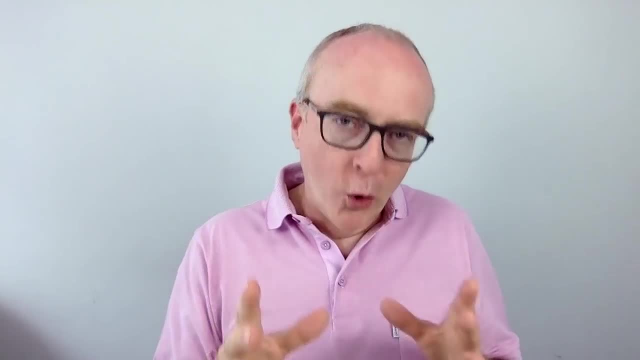 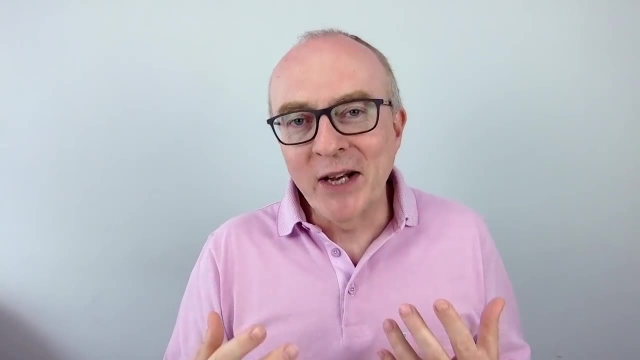 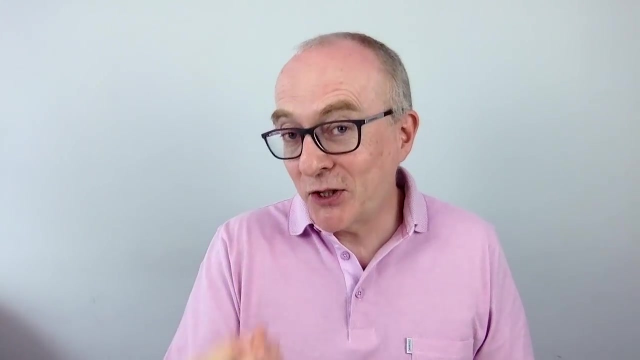 think the last one is a more effective communicator. Not always right, I know. it depends on the context and who you're speaking to, but generally speaking, the eye contact, having some eye contact, a pleasant manner and smiling make you a more effective communicator, And it's especially 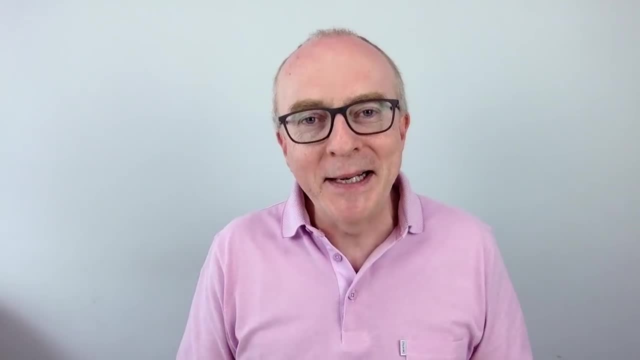 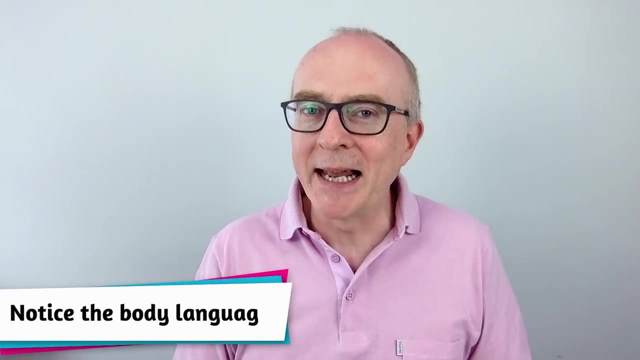 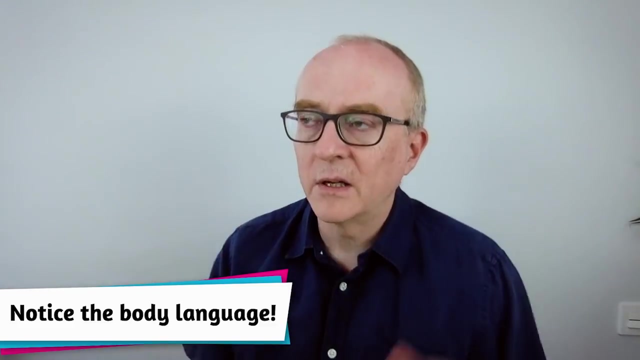 true in interviews, job interviews, IELTS speaking tests. Let's go back and listen to the first speaker of this video and notice the body language. If I had a lot of money, I would purchase a majestic mansion on the rocky coast. 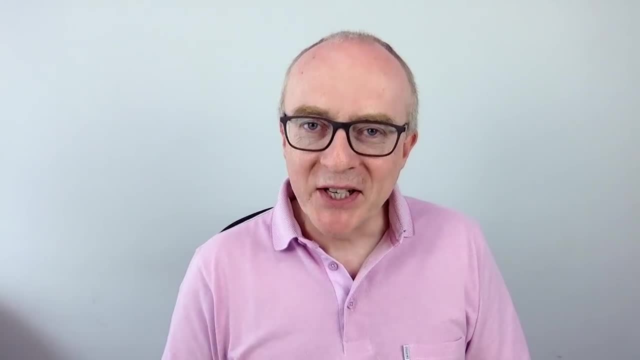 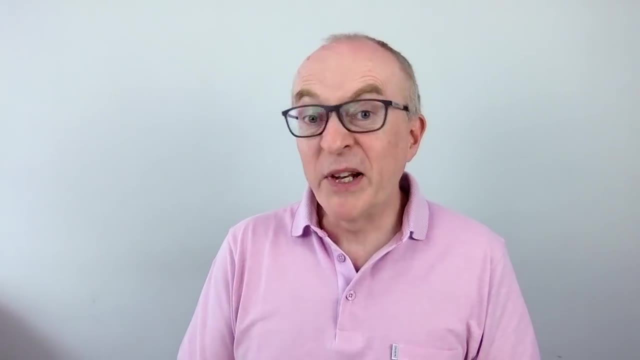 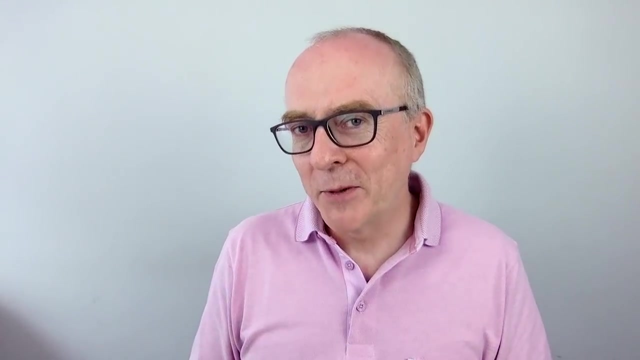 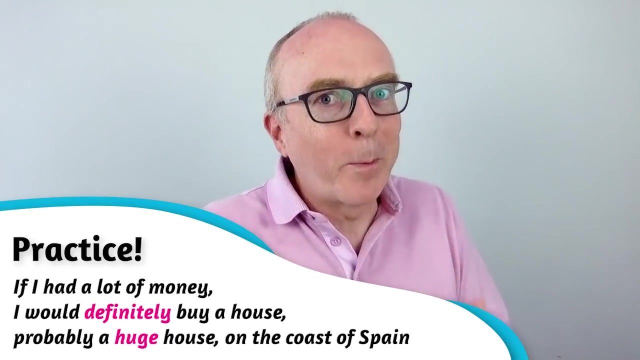 First lines of Spain. Now let's see if I can improve it. If I had a lot of money, I would definitely buy a house, probably a huge house, on the coast of Spain, right? More powerful communication- Great What you can do now: practice yourself, Take the words, try and use your body. 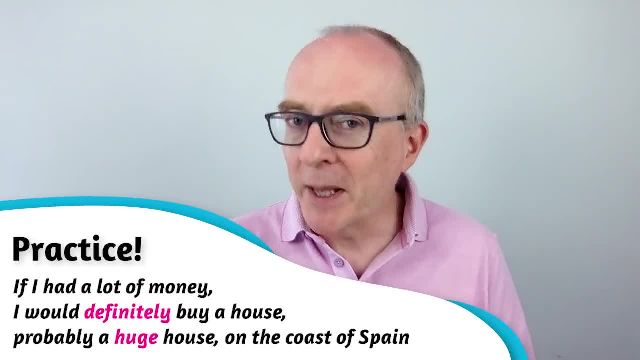 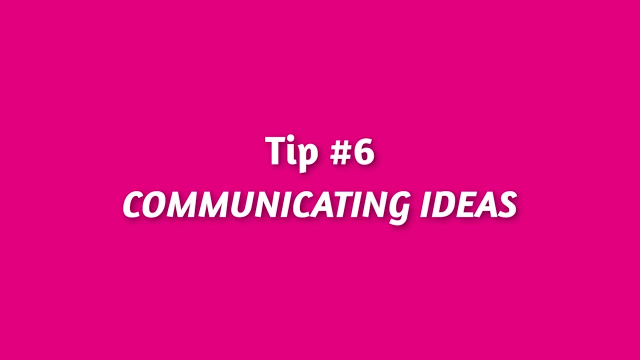 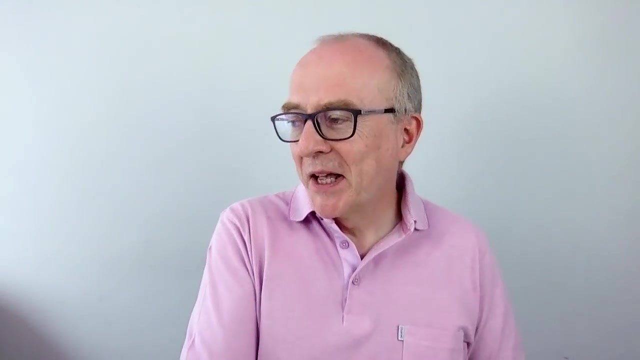 language, eye contact, manner, smiling, to be a better communicator. Have a go, That is great. Keep on practicing while we move on to tip number six. So tip number six is about communicating ideas. Communication is all about getting your ideas across. So if you're a communicator, you need to be able to communicate your ideas across. 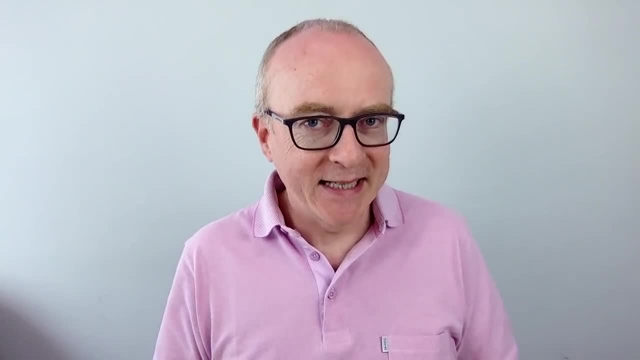 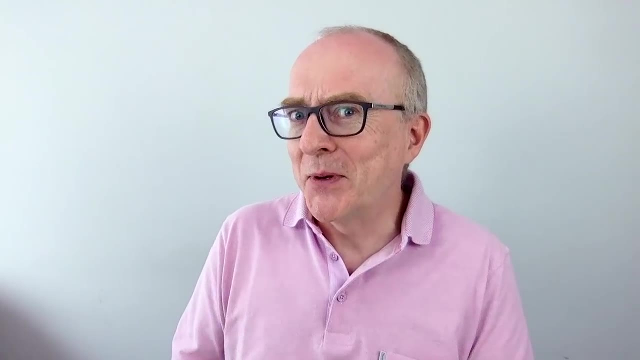 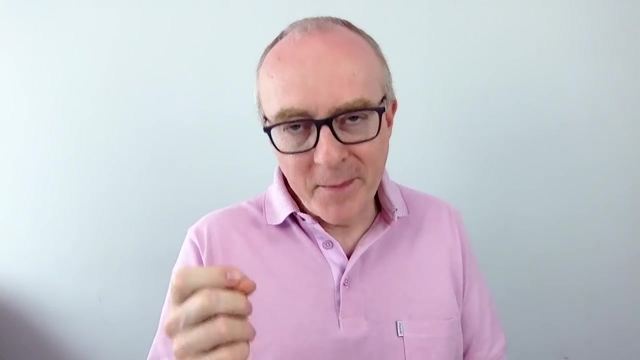 It's not about speaking perfect English In order to communicate ideas. well, of course, you need to have ideas to communicate. If you've got no ideas, then there's no communication. But this is a common problem for many students And they ask me: Keith, what do I do in IELTS? 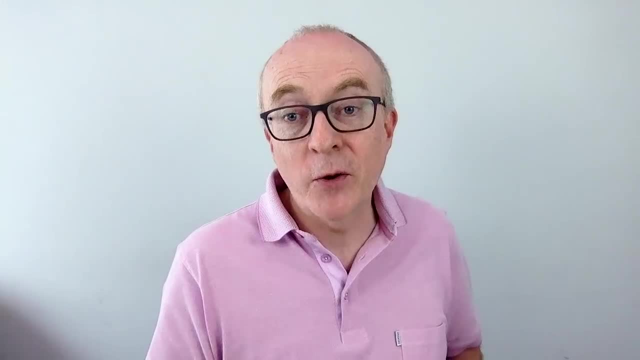 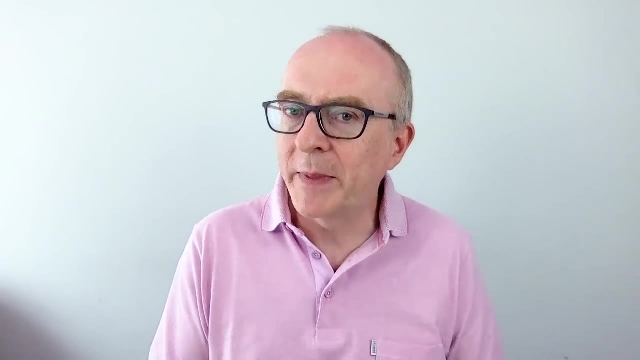 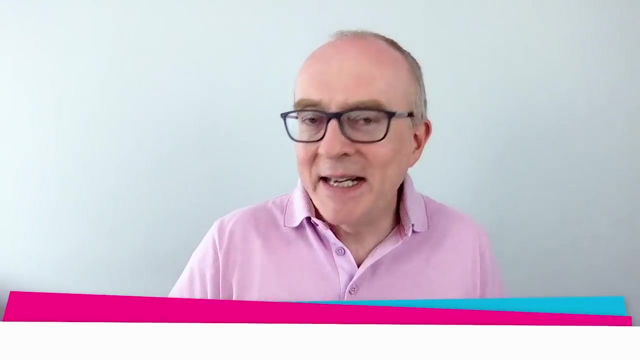 speaking if I have no idea about the topic. Well, of course you can say one or two clever things like: well, I haven't thought about that before, But you know it's not very effective. What you really should be doing is reading and listening to a wide range of material. 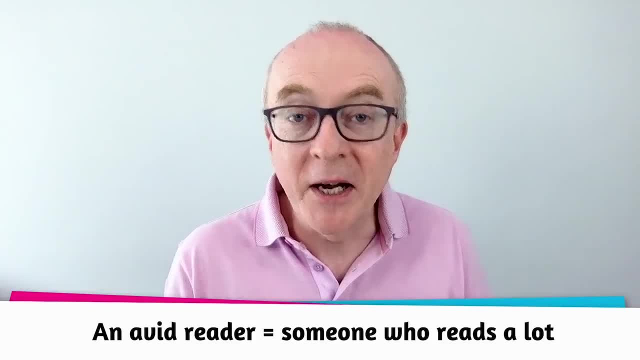 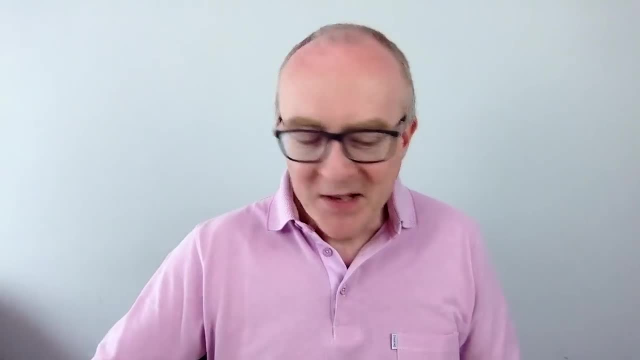 on different topics. Become an avid reader. Start reading books- books about food, maybe. books about Edward Snowden. Read magazines, right? Maybe news, maybe others. Read some interesting websites. Read some interesting books. Read some interesting books. Read some interesting books. 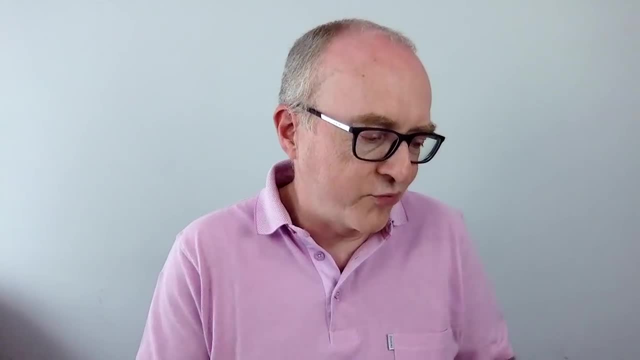 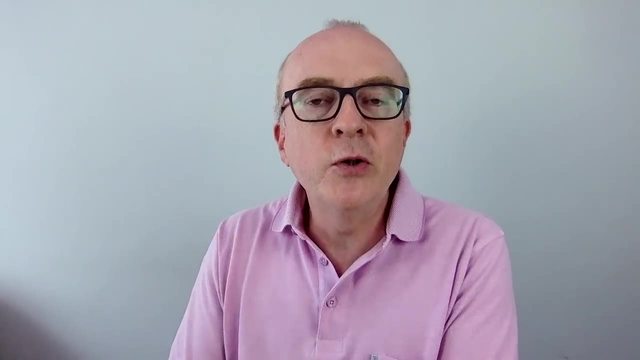 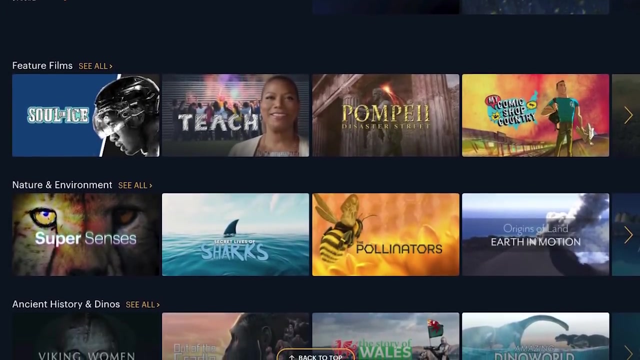 Check out this one, The Conversation- Brilliant website. Lots of interesting ideas Also be watching things- videos, I mean. you can go to YouTube. I would recommend CuriosityStream. right For under $20 a year, you get access to a wide range of amazing documentaries. 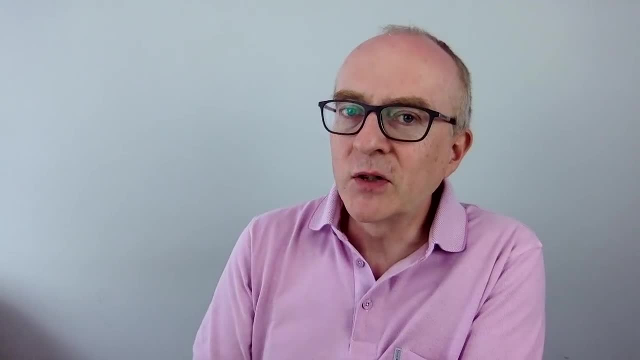 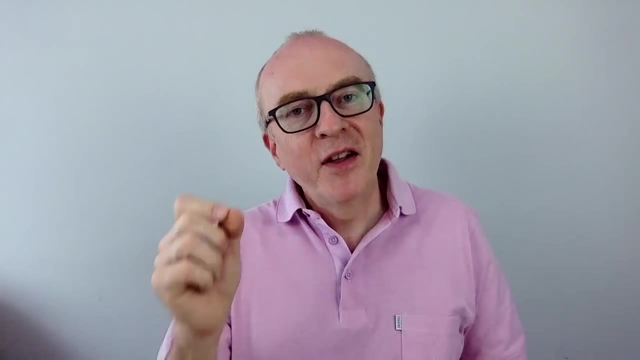 films, very specific topics, really useful for ideas? Yes, Another thing you can do is, if you've got a lot of ideas, you can go to YouTube. Another thing you can do is to be asking yourself this question every day: What do you think of? 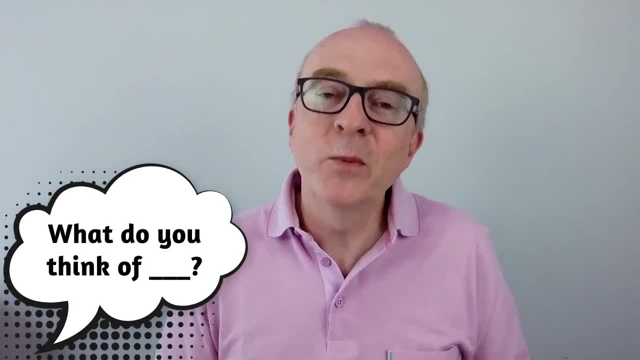 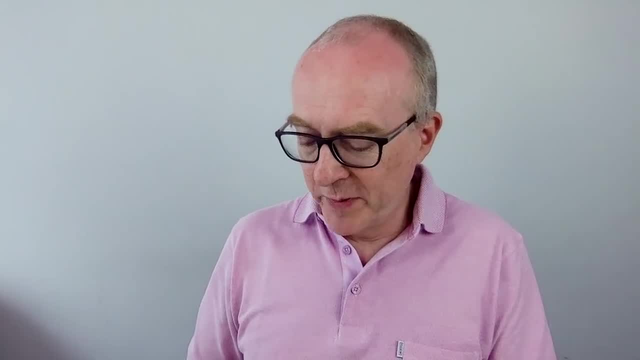 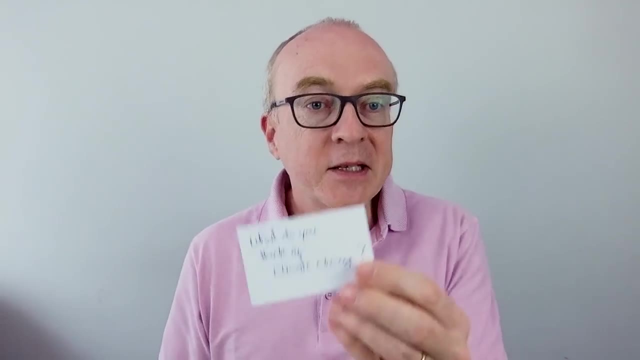 Right, Ask yourself that question. I, even in other languages, write little cards, right? I mean, I'm a bit of an old-fashioned person- Call me an old fogey if you will- But I like flashcards where I write them down. So I may write down things like: what do you think of climate change? 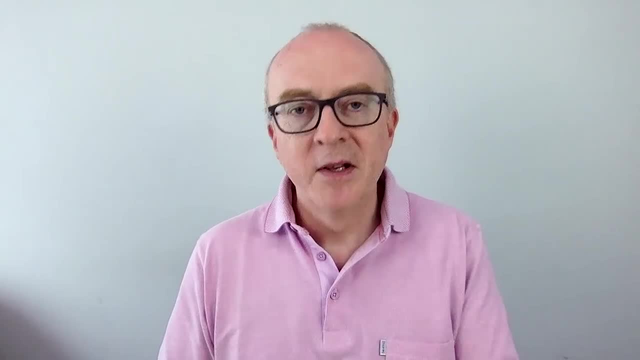 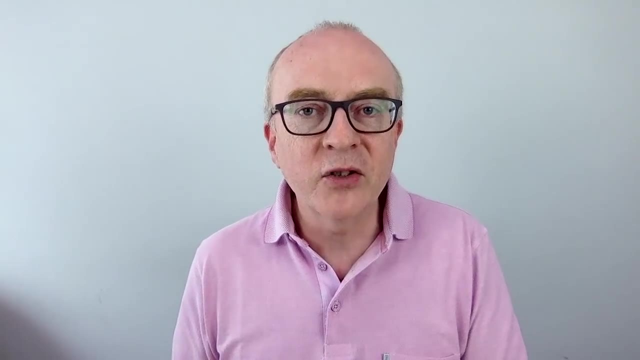 What do you think of Artificial intelligence? What do you think of science? And just each day, I'll just pick up one and I'll start answering, And if I can't get an answer, I'll go and read something that can help. 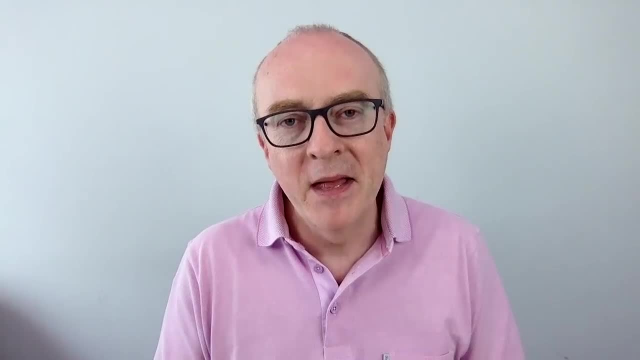 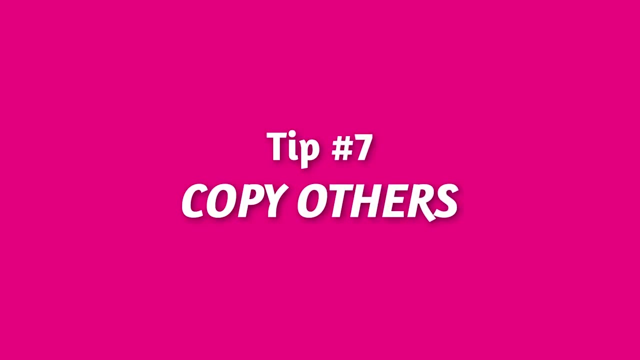 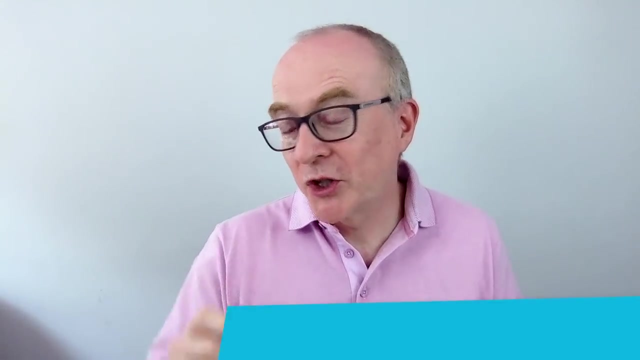 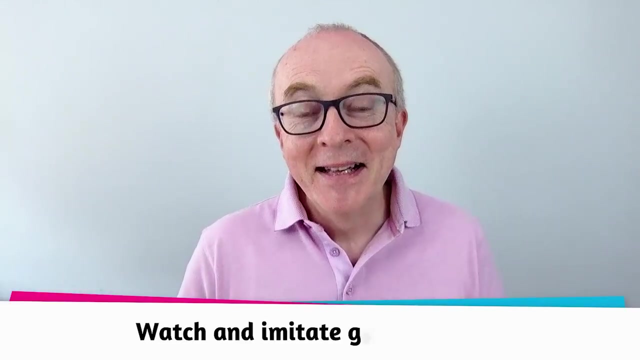 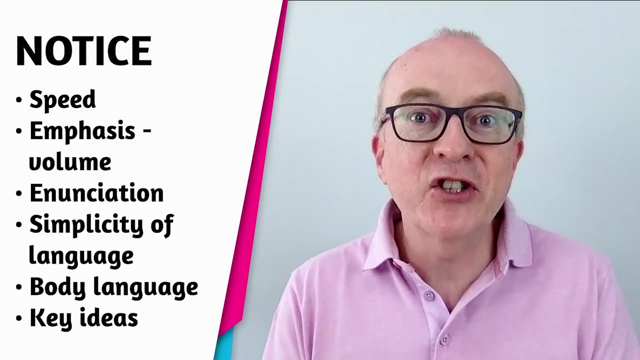 me get some ideas about it right. Become an avid reader. Great, Let's move on. Tip number seven: copy others. I recommend that you watch some great speakers and communicators right And copy or imitate everything they do. Watch them and notice the speed, the emphasis, volume, enunciation. 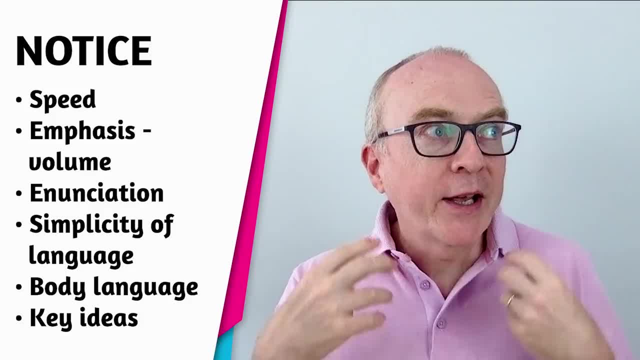 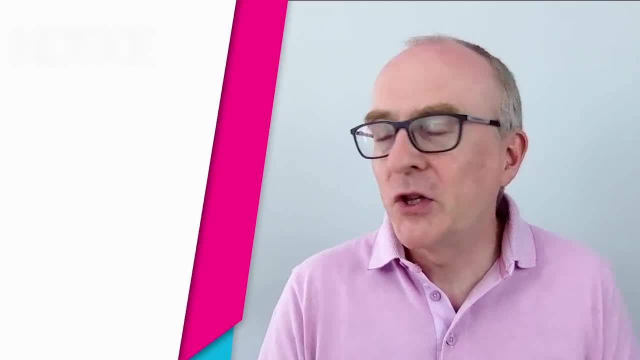 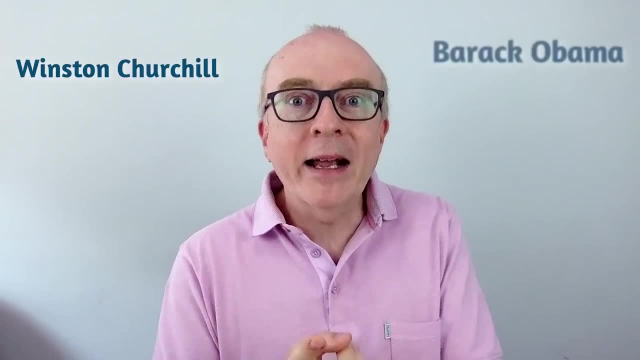 simplicity of language, body language, getting their ideas across right. Watch them and notice these things and then copy them. You may, you know, you may want to look at a lot of other things. people like I don't know, I mean some people say Winston Churchill, possibly Barack Obama. 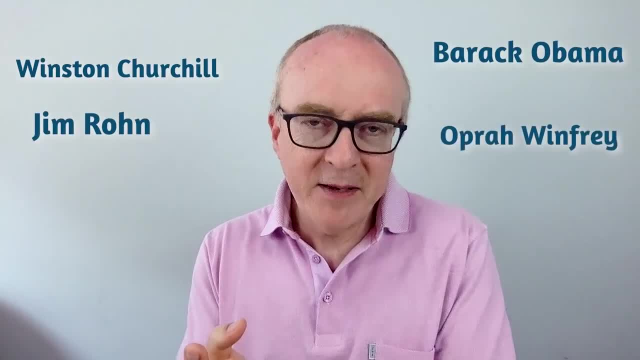 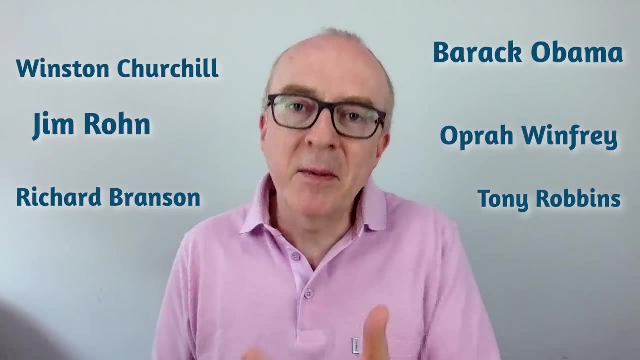 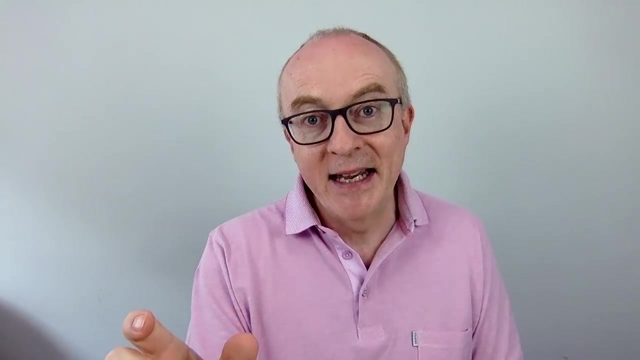 for sure. Jim Rohn, Oprah Winfrey, brilliant Richard Branson, another great one, Tony Robbins- not everybody's cup of tea, but maybe Just go and watch them. In fact, what you can even do is just take two or three sentences that they say right, Break it down and try and imitate. 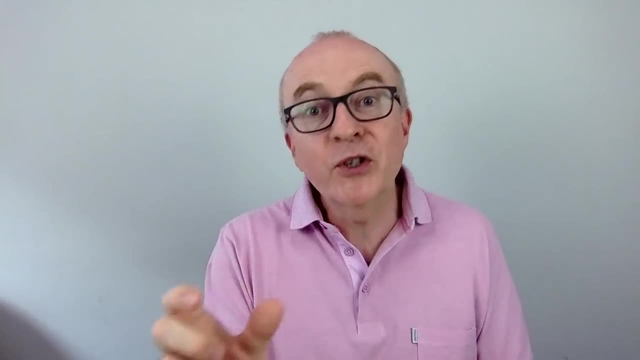 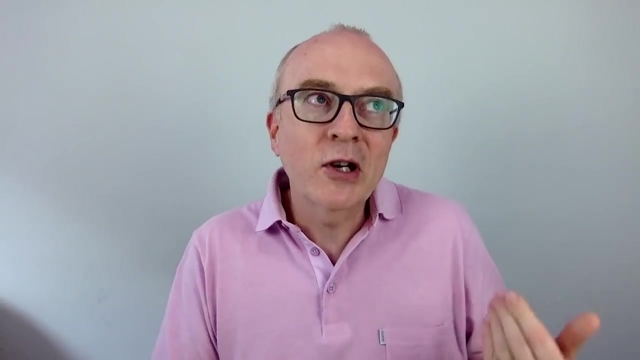 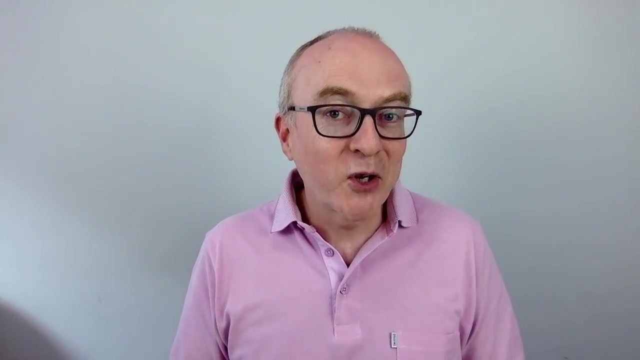 exactly what they say, Just for two or three sentences. Record yourself, Do this over several days and to see how you get closer and closer to being just like them. It's a great exercise to do. Help build up your confidence, as well as communication skills. That's it. Oh, there's still a bonus. Let's go over to. 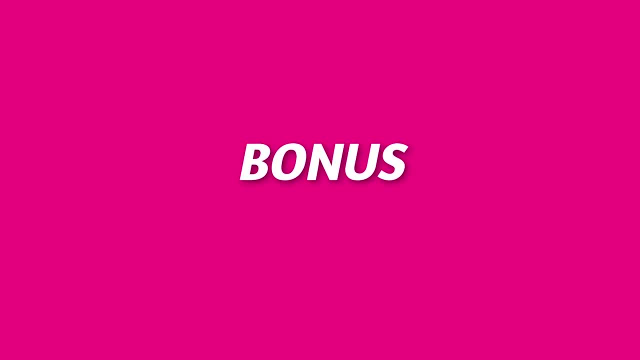 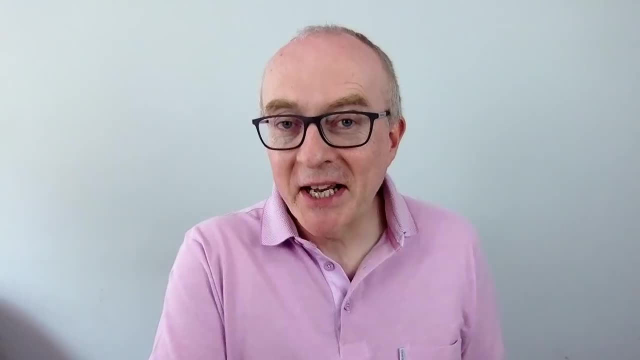 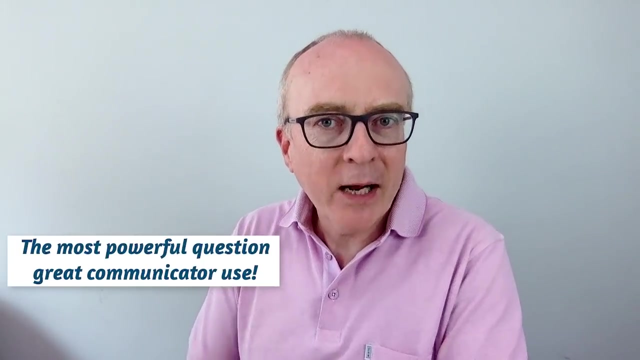 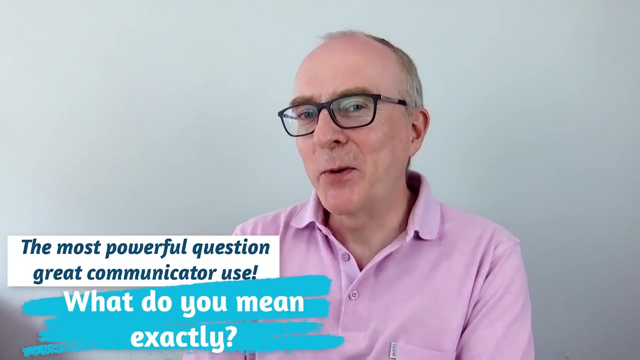 that bonus. So, if you remember, at the beginning of the video I did say I would tell you the most powerful question that great communicators use. So that question is: what do you mean exactly? It's a great question. It's a great question because it makes the other 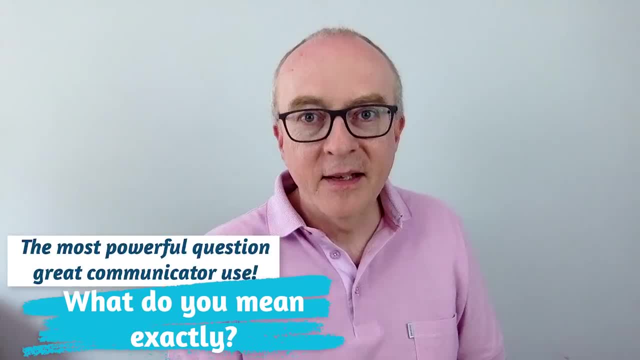 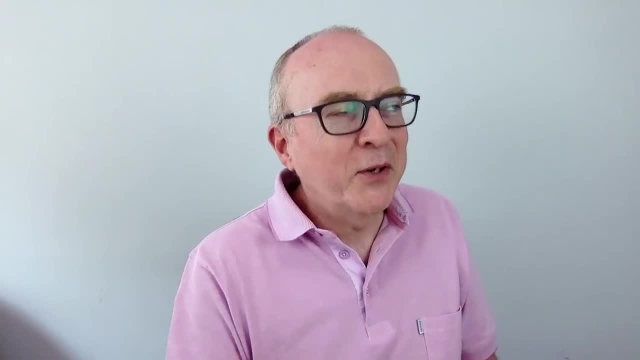 person think that you're in a relationship with them. It's a great question because it makes the other person think that you're interested in them and their ideas, because you're asking them to clarify it- And maybe you are- but also it helps build trust because they think you're interested. 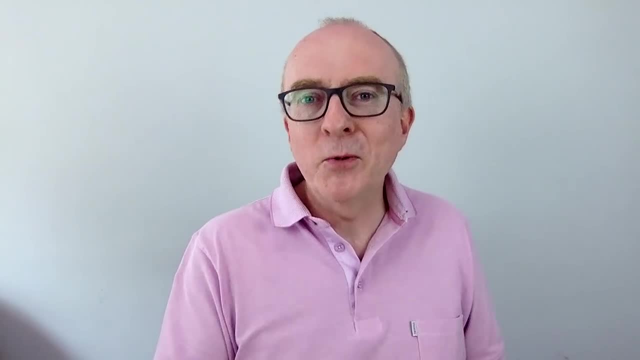 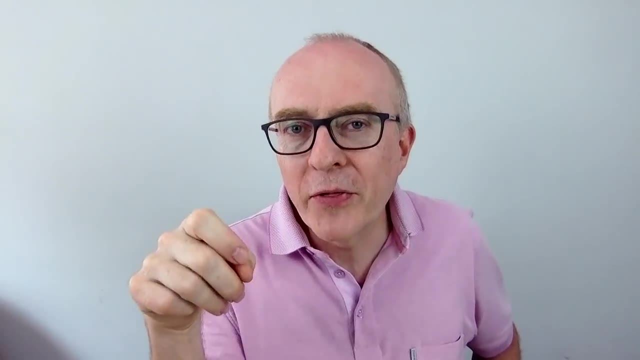 You're trying to listen, understand them better. So it builds trust. It's great In IELTS speaking. it's a great question because if, especially in part three, you don't fully understand something or you're not sure, you just say: what do you mean? 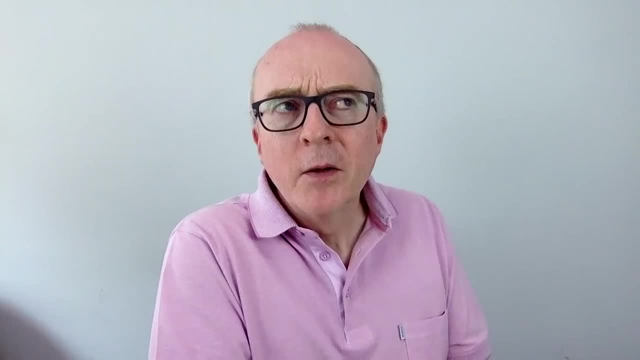 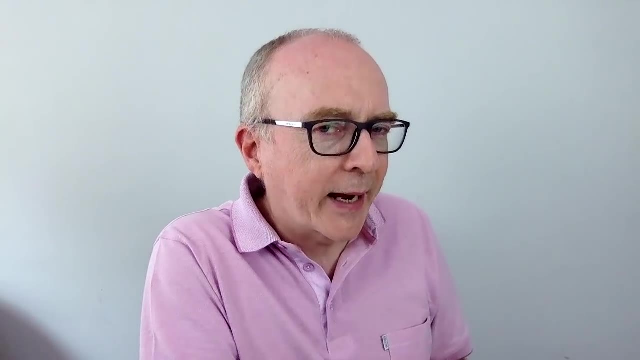 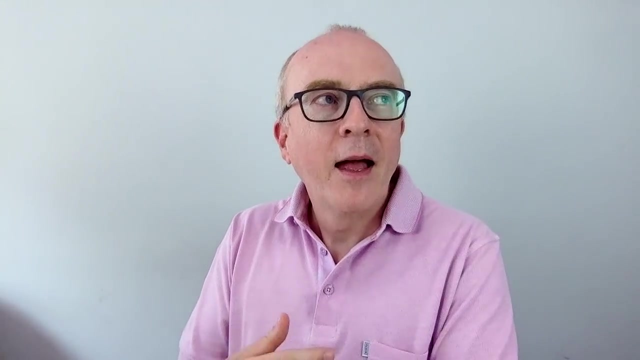 Exactly. You know, if the examiner says: well, do you think consumerism has overtaken our society, What do you mean exactly? Well, do you think that people buy too many things? Ah, okay, And then you give your answer right. It's a great question to build trust. 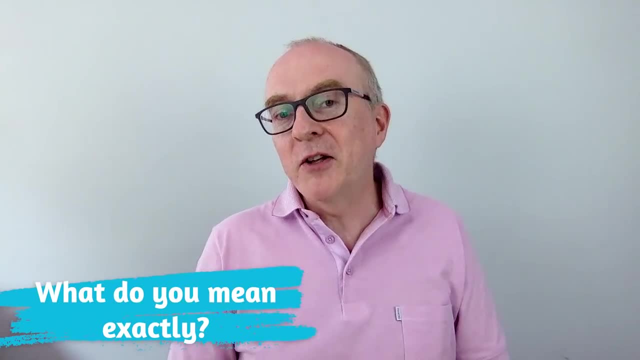 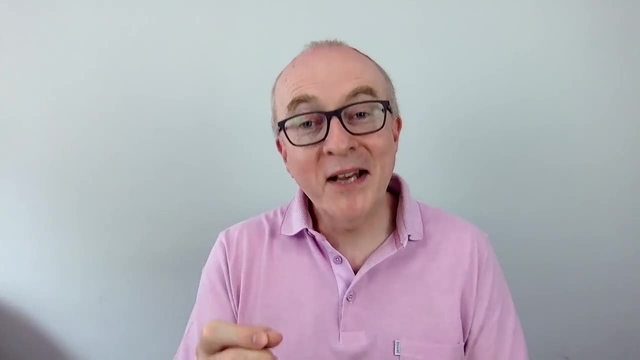 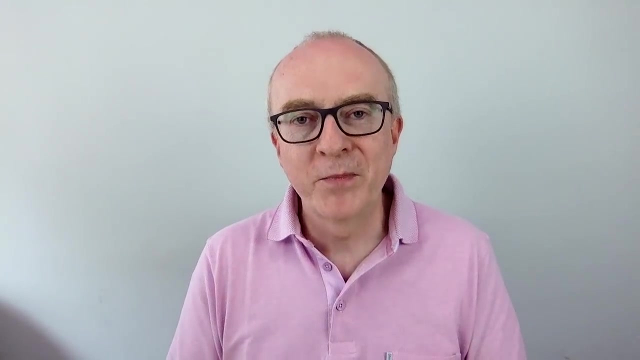 to help you become a better communicator, not just in IELTS speaking, but in any kind of conversation. Fantastic, That's it. I hope this helps you see that good communication is not just about good English. It's so much more. Communication is a skill that you need to develop, and it takes time. 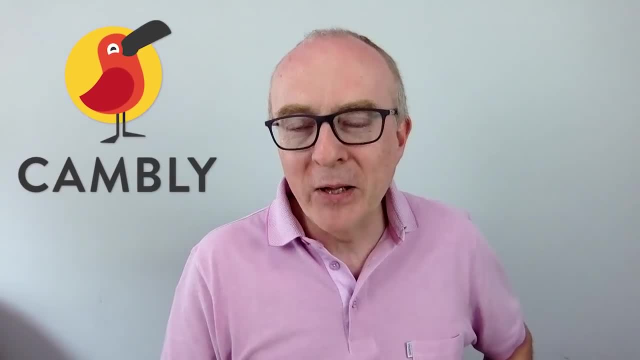 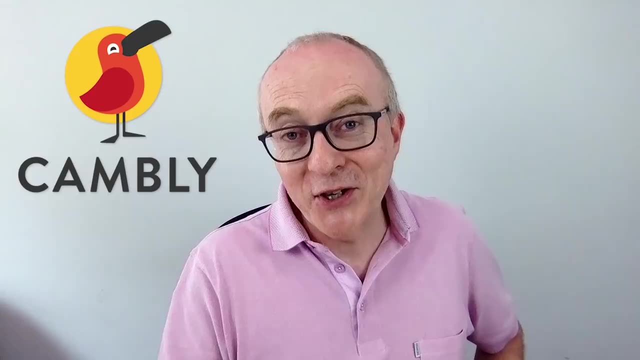 Remember, go and check out Cambly, where you can practice and build up your communication skills with native English speaking teachers. Also, if you're a first-time user, you can take a 10-minute free lesson to check it out. And if you're a first-time user, you can take a 10-minute free lesson.